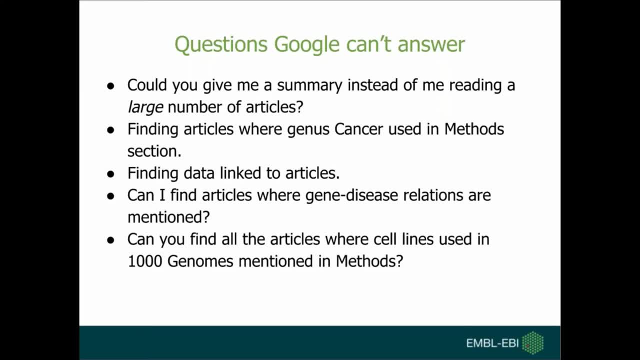 This is what Google can add to, And sometimes you want to find articles where helping også nängt grieving cancer used in methods sections And other examples that are finding articles where, compared with Medicine papers and other things in your detailed archive, are much better. 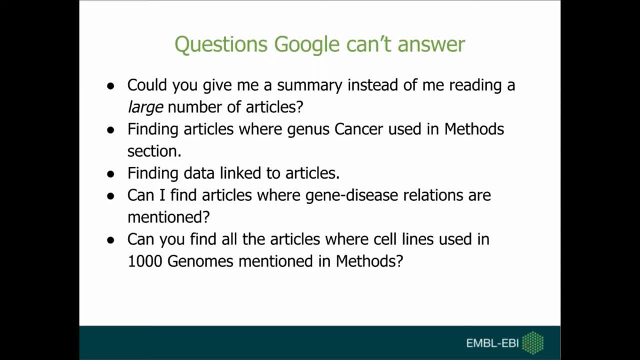 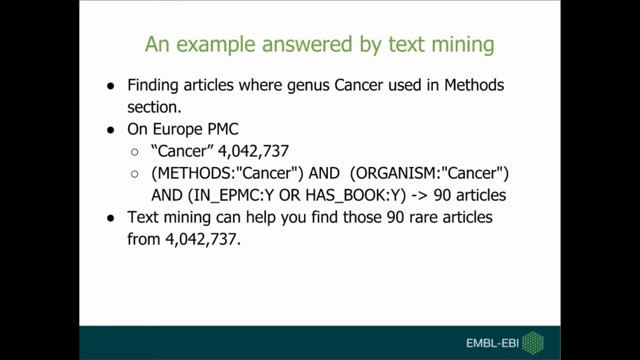 where data is used and mentioned and especially with links to get those data. So these are questions where using Google cannot answer questions And, for example, this is one good example where text mining actually can help you. So let's go back to the example I mentioned, where, if you want to find all those articles, 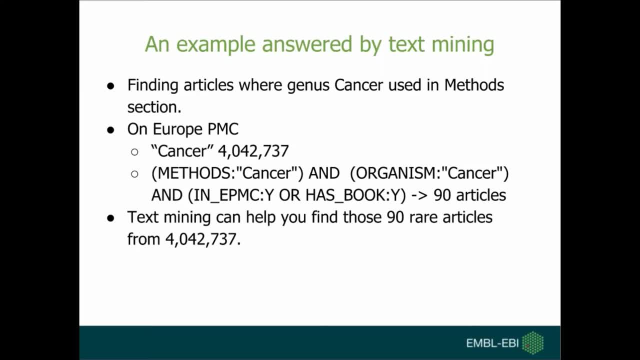 where genus cancer, not disease cancer, is mentioned in method section On Europe PubMed Center website. if you just search for cancer, that will give you around four million articles. If you can make a query where you can specify, OK, I want to find cancer specifically mentioned. 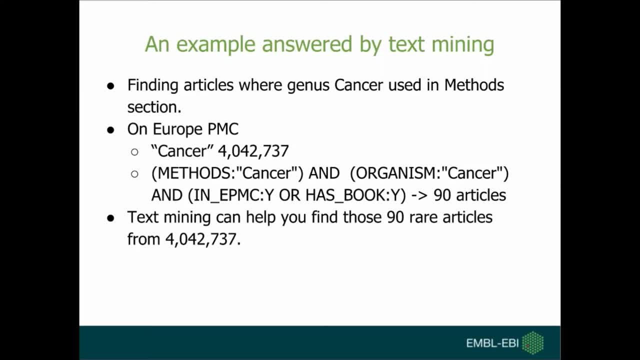 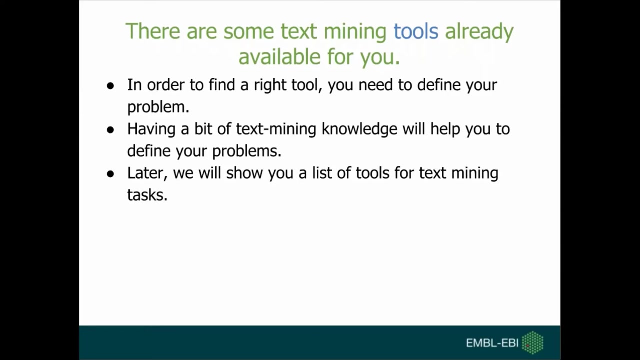 in methods and organisms which are organisms, then it will give you only genus cancer, Only 90 articles. Text mining really can help you to find those 90 real articles from one million articles. So there are already some text mining tools already available for you. 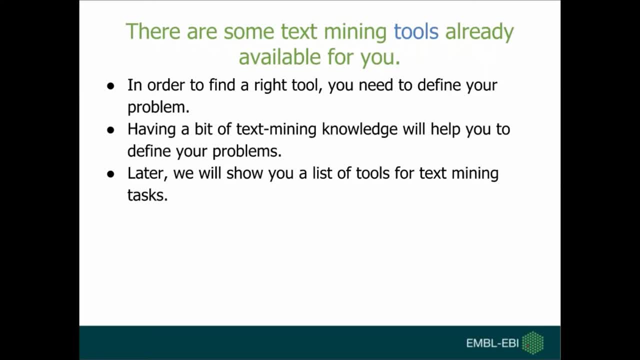 But in order to find a right tool you need to define your problem first, And having a bit of text mining knowledge will help you to define your problems. On next slide we will explain what is text mining and what kind of problems in text mining. 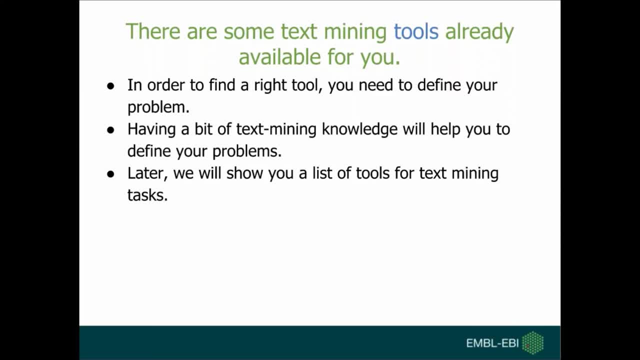 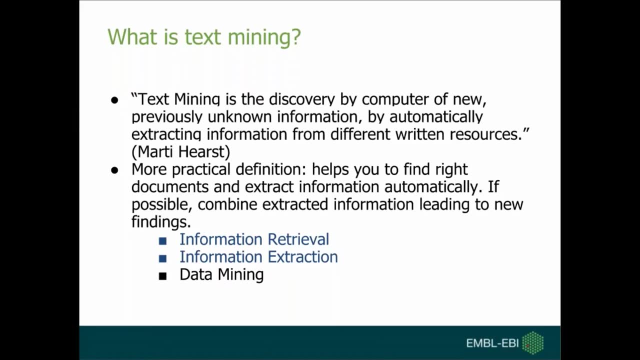 which help you to find relevant tools for your problems. So what is text mining? According to Marty Hurst, text mining is the discovery by computer Computer of new, previously unknown information by automatically extracting information from different written resources. More practically, this means text mining can help you to find right documents and extract. 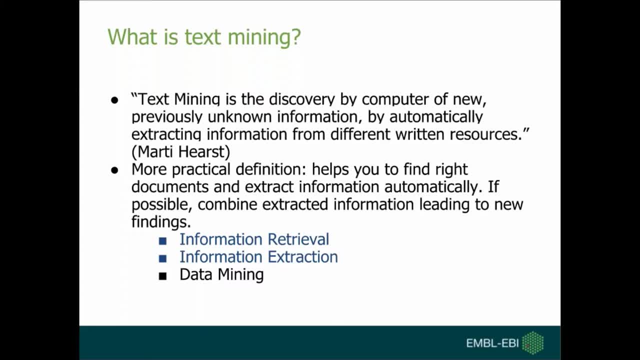 information automatically And, if possible, you can combine those extracted information which leads you to find new findings. The first part is information Information retrieval, which will help you to find right articles and extracting information. The second part is information extraction, where you can extract information in a large 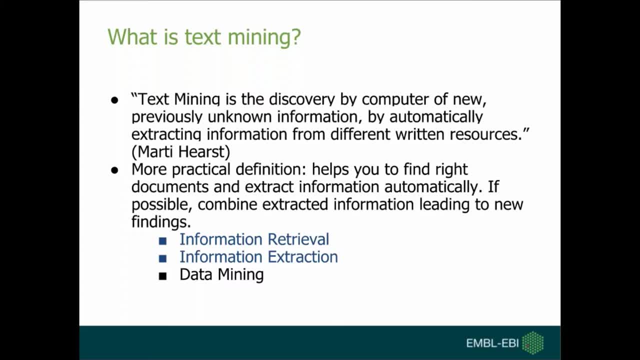 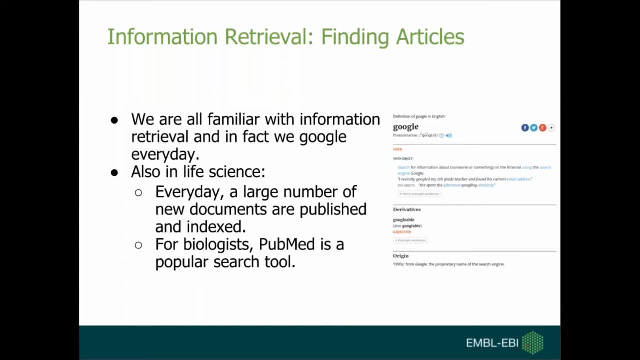 scale. So we will focus these two parts in the next slides. First, information retrieval is to find relevant articles. You are all familiar with information retrieval And in fact you Google every day. Also in life science, every day a large number of new documents are published and indexed. 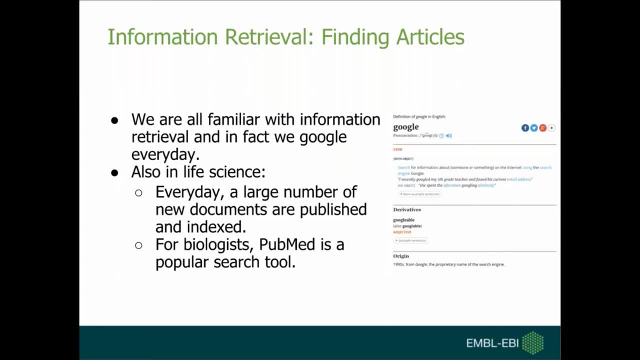 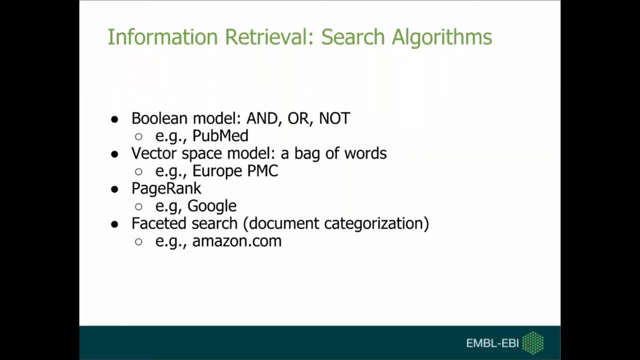 And PubMed is, for example, one of those popular search tools for biologists. Search algorithms In information retrieval: there are several search algorithms, such as Boolean model, vector space model, PageRamp, And there are several search algorithms. There are several search algorithms, such as Boolean model, vector space model, PageRamp. 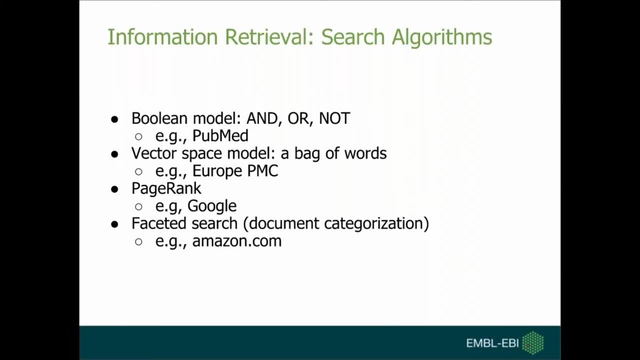 And there are several search algorithms, such as Boolean model, vector space model, PageRamp, Which is a facade search, which is more like document categorization, And the reason I'm introducing this subs Mentioning these algorithms is knowing search algorithms behind the site you are using is. 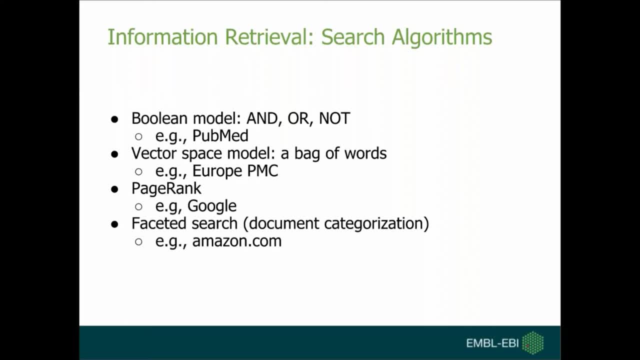 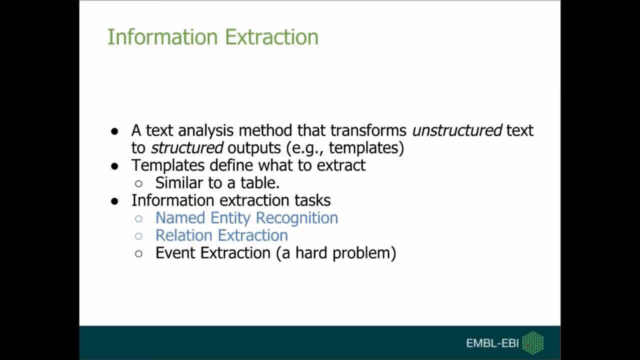 important because that makes you understand search result returned by those subs engines. Information extraction is a text你就11. analysis method that transforms unstructured data to structured outputs. At first you have to define your own templates which basically tell you what to extract from articles. This is very similar to a table Information. 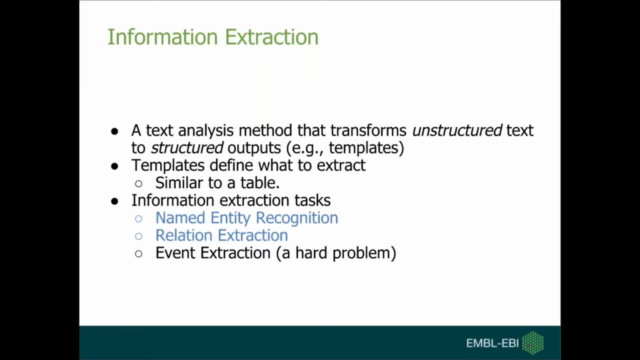 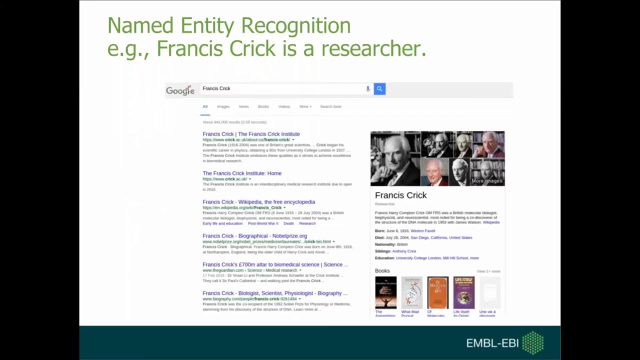 extraction tasks consist of many three tasks: named entity recognition, relation extraction and event extraction, which is the most complex and or hardest problem. In this presentation, we're gonna only focus on the first two: named entity recognition and relation extraction. So what is named entity recognition If? 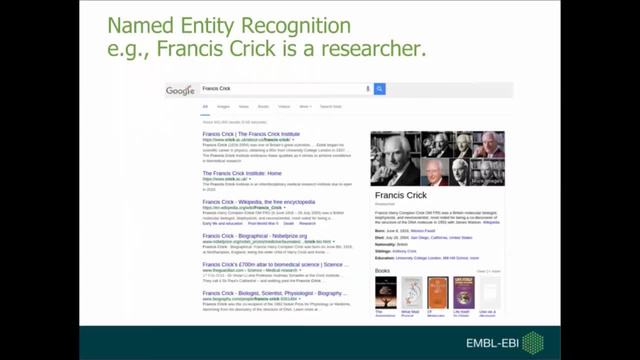 you search for Francis Crick on Google besides retrieved pages, Google algorithm recognizes a Francis Crick as a name. So if you search for Francis Crick on Google besides retrieved pages, Google algorithm recognizes a Francis Crick as a name name and provides more information on him. 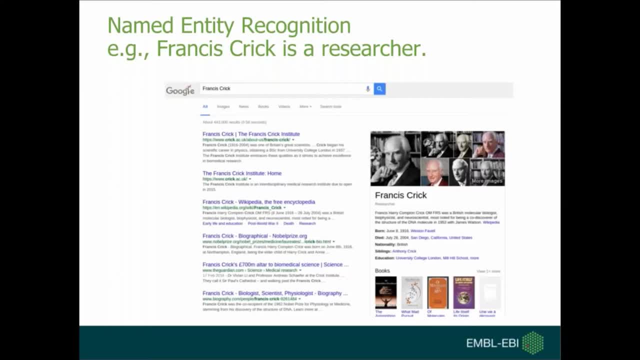 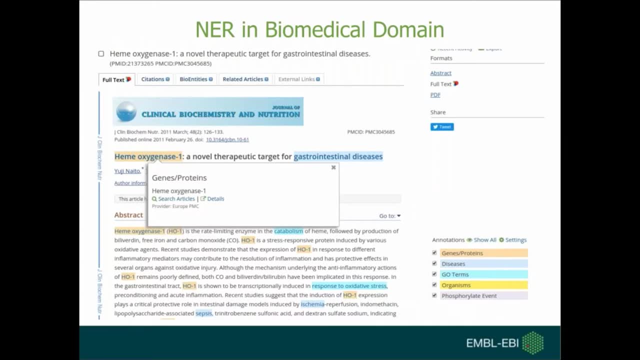 This is one good example of named entity recognition. In biomedical domain, gene, protein, disease organism and chemical names are important and these names can be recognized by text mining algorithm. For example, Hemoxygenase 1 was recognized and linked to Uniqlo for more information. 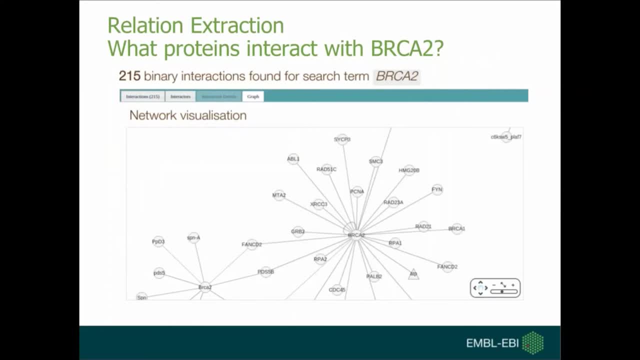 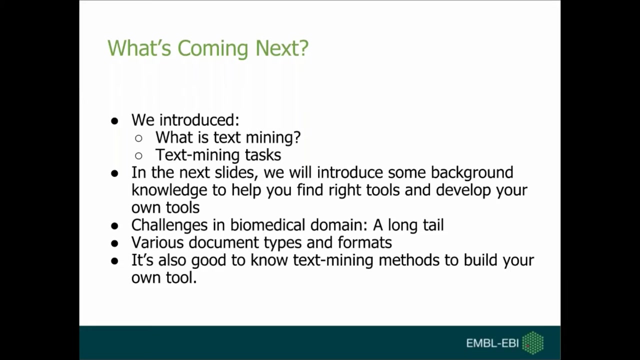 on this website. Relation extraction. Another task of information extraction is relation extraction and its task is to discover semantic connections between entities. For example, given a protein, BRCA2, finding all the proteins interacting is a relation extraction problem. So far we introduced what is text mining and text mining tasks. 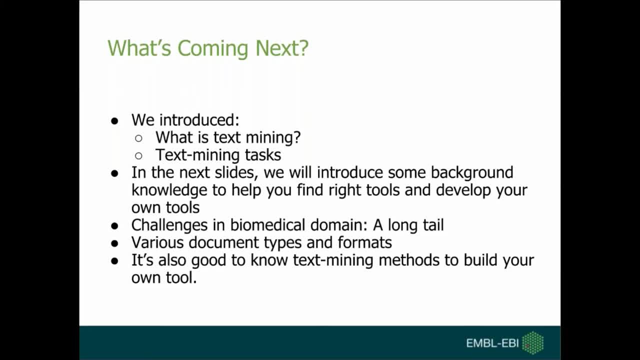 The next slide will introduce some background knowledge which can help you to find right tools and develop your own tools. In order to build your own tools, you should know what text mining means. The methods are available For that. my colleague Şenay will continue to explain what are those methods. 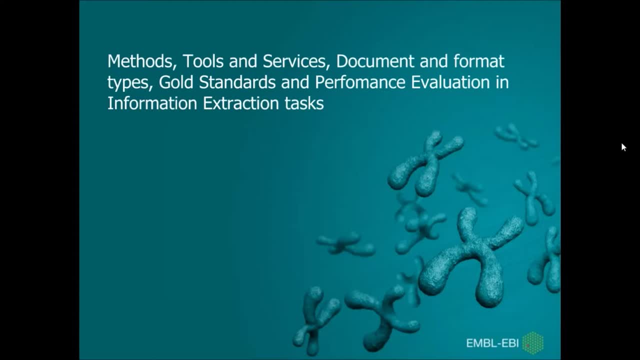 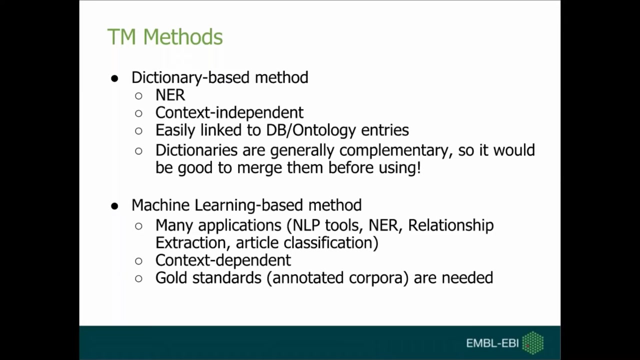 In this part, I will talk about methods, tools and services, document and format types, code standards and performance evaluation used in information extraction tasks. There are four different methods used to develop text mining tools for extracting information. One of them is dictionary. 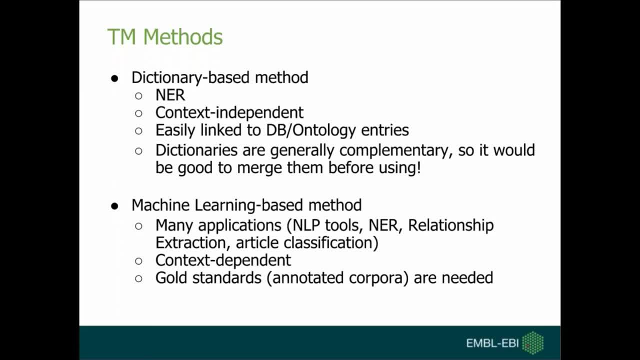 It is a dictionary-based method. This method involves in creating a dictionary from terminological resources and using it for name entity recognition problems. It's a context-independent approach. By using this method, it is easy to link annotated entities in text to dictionaries or ontologies. 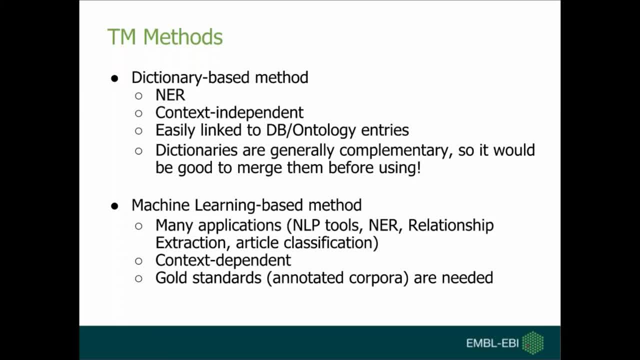 Previous studies utilizing dictionaries revealed that dictionaries are generally complementary, so it would be ideal to merge them before you use them. There are three ways to do this. The first is to use the dictionary. The second, to use the dictionary. The third, to use the dictionary. 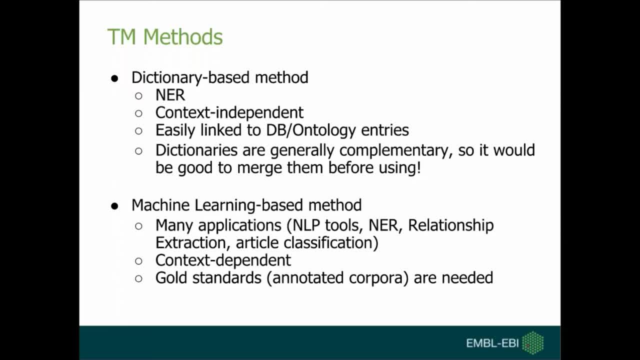 using. Another method is machine learning. This method can be applied to various text mining tasks, such as name, entity recognition, relationship extraction, article classification, as well as developing natural language processing tools, for example a POST tagger. It involves in training a learning algorithm on a. 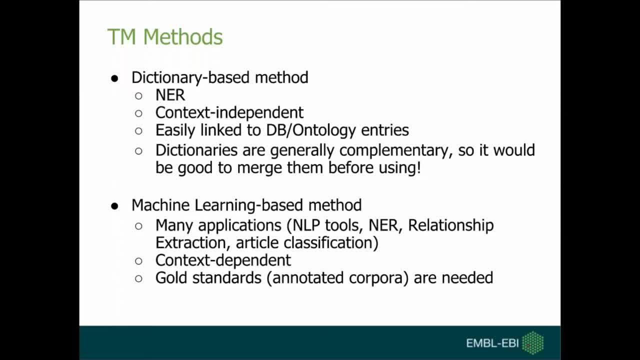 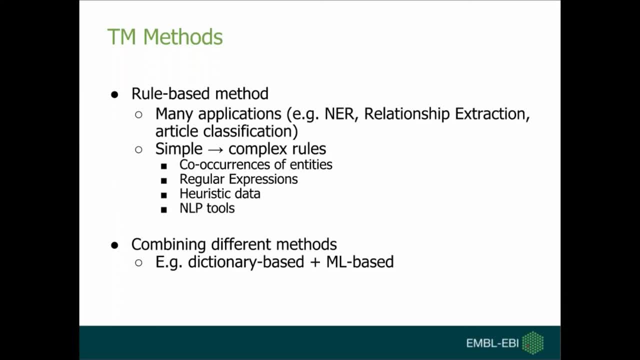 gold standard data set and therefore it's a context dependent approach. Similar to machine learning method, rule based method can also be applied. many problems, such as name, entity recognition, relationship extraction and article classification, Rule based system vary from simple to complex, depending on the 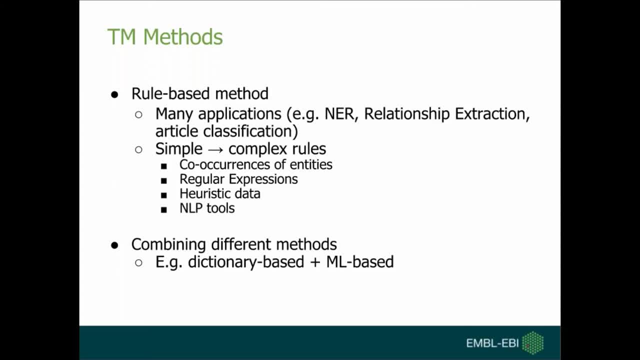 complexity of the rules used to implement this system. For example, a system utilizing concurrences of entities for extracting associations would be the simplest approach, and utilizing regular expression, heuristic information or natural language processing tools would make the system more complex. It is also 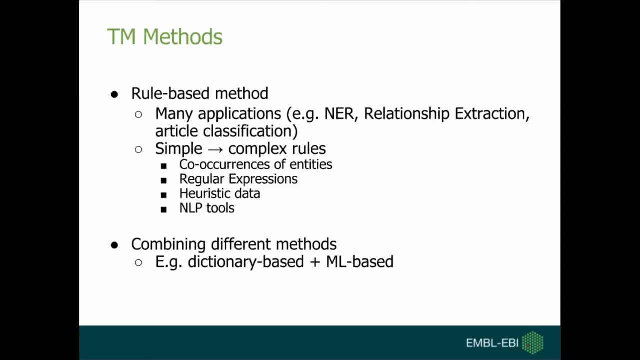 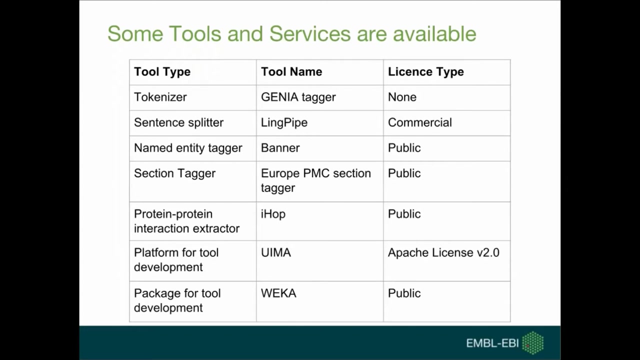 possible to combine the three aforementioned methods and create a hybrid system. for example, a machine learning base in addition to a dictionary-based method can be used in combination in name entity recognition tasks. There are various tools and services publicly or commercially available for either direct use or developing new text mining pipelines. 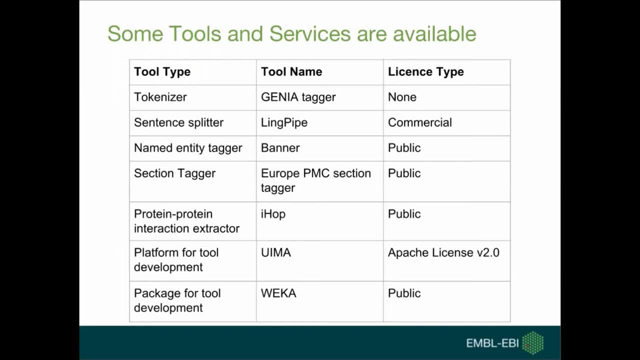 One such tool is GeniaTagger, which splits a given text into its tokens. Tokenizer is a natural language processing tool, and it can be used for the development of other natural language processing tools, such as sentence splitters, as well as name entity. 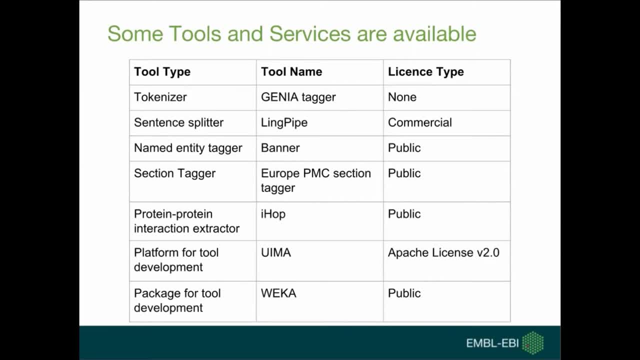 recordinizers and classifiers. Another one is a sentence splitter called link pipe. Determining sentence boundaries is very important, especially for relationship extraction tasks. Banner is a name entity recordizer and EuroPMC section section tagger is a tool that can identify different sections of a given full-text article. 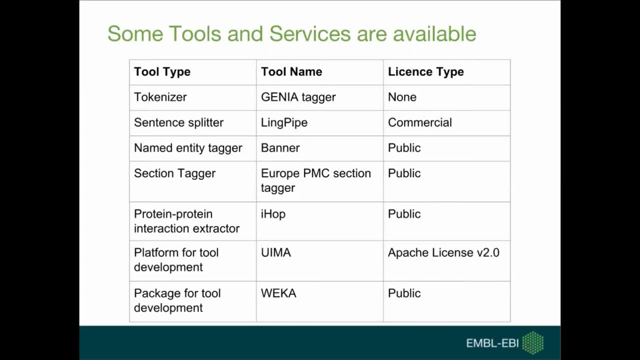 IHOPE is a text mining service that can be used to extract and visualize protein-protein interactions. There are also platforms that can be used for developing text mining pipelines. UEMA is one of them, and there are some packages that can be used to develop machine learning-based. 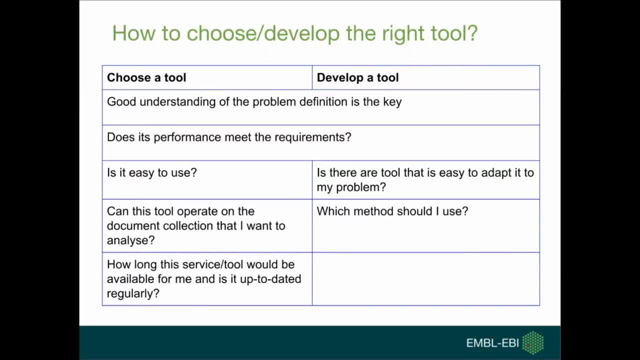 text mining tools such as WEKA. There are many tools available for using and developing new text mining systems in case needed. However, one important question to answer is how to choose or develop the right tool. There are a couple of points that we need to consider before attempting to use or develop. 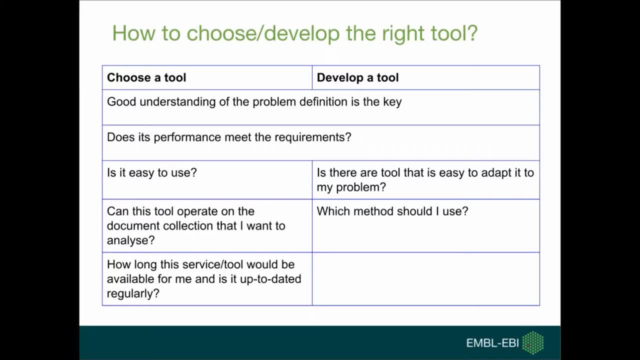 a tool. These are shown in the table. Independent of whether we attempt to use or develop a tool, we need to consider whether we use or develop a tool. Firstly, we need to have a good understanding of the problem definition and ensure that its performance meets the requirements. 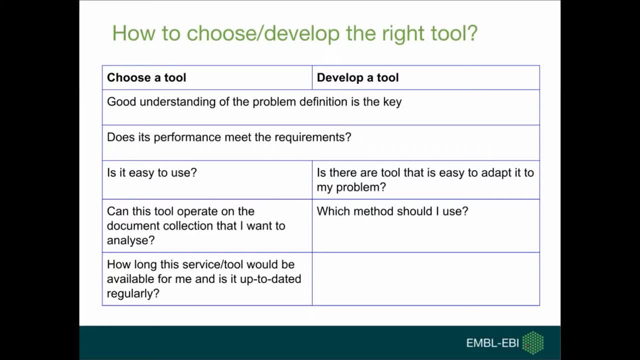 If we intend to use an existing tool, we should check whether it is easy to use, operates on the document collection that we think contains the information that we look for, provides up-to-date results and available for a long enough period for us. 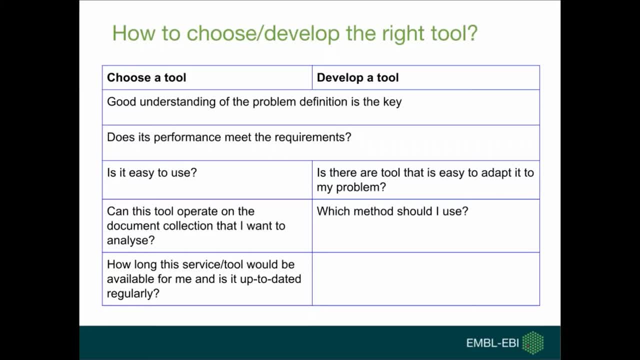 There are a number of tools that we need to consider before attempting to use or develop a tool. If we intend to develop a text mining tool, then first we should check the available tools to see if there is any that we can adapt to our requirements easily. 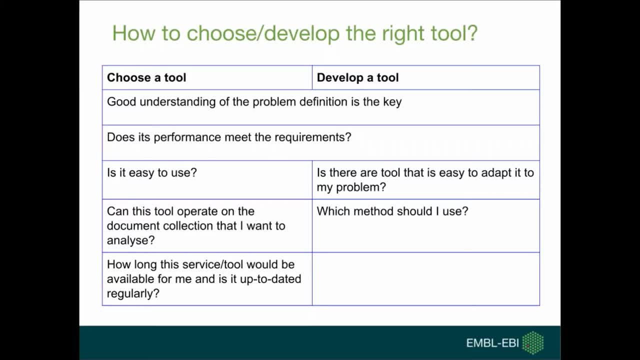 Otherwise, we should choose carefully a suitable implementation method among the ones that I mentioned earlier. Choosing an implementation method depends on the problem definition. For example, if you are a protein-protein interaction creator and would like your text mining tool to bring you all the possible protein-protein interactions for your further 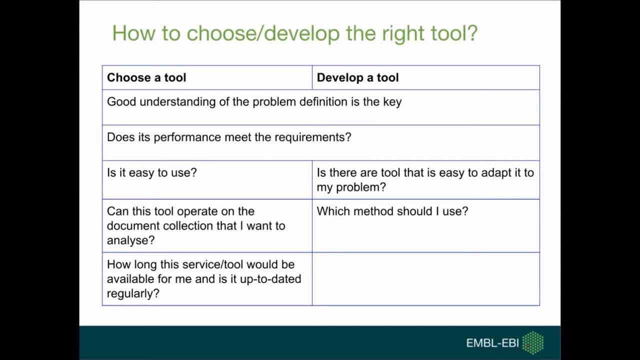 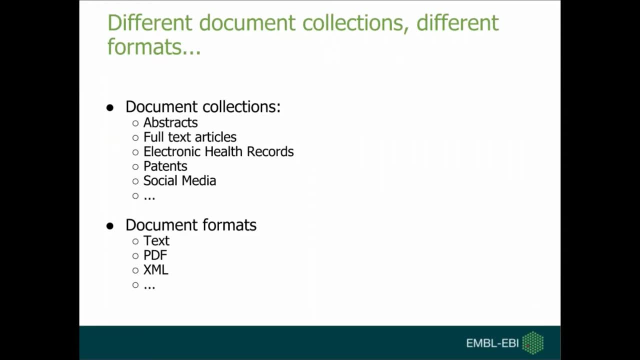 manual analysis, you could develop a recall-driven, rule-based system operating on the co-occurrences of proteins at the sentence level. As I mentioned in the previous slide, document collection type and format play a role in the tool selection, Document collection and development. 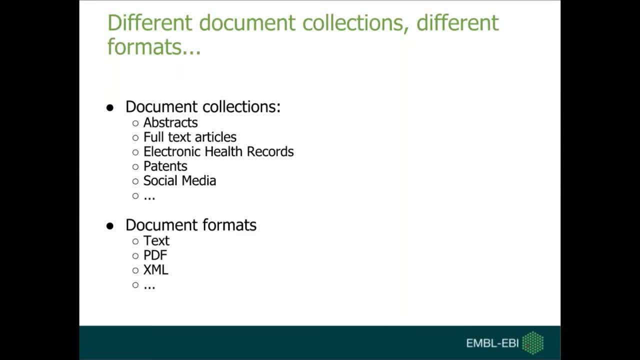 There are various document types, such as abstracts, full text, electronic health records, patents and social media. Documents exist in different formats, such as text, PDF and XML. We should do a little bit investigation in order to understand where is the information. 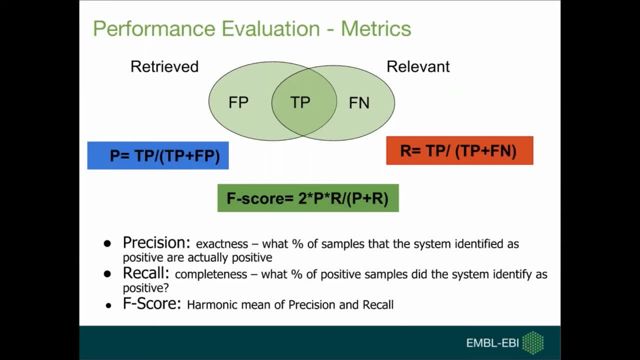 that we look for is buried and in which format. Performance evaluation is an important issue For tool usage and development. there are three commonly used metrics for evaluating performance of a text mining tool. These are precision, recall and F-score. We can explain how to estimate these values based on an example. 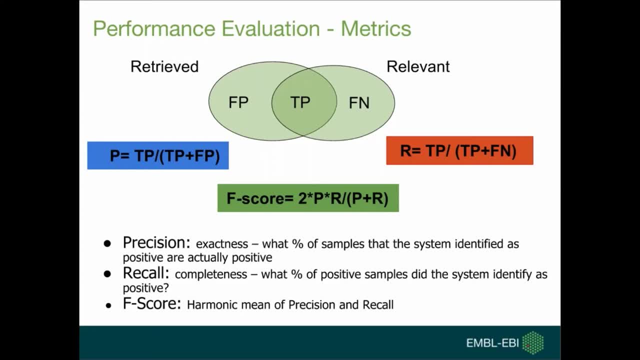 Suppose there is a text mining tool which retrieves relative documents based on a specific user query from a pool of documents. Obviously this is not an easy task. It takes a lot of time. Obviously, the document pool contains the actual relevant documents to the user query. 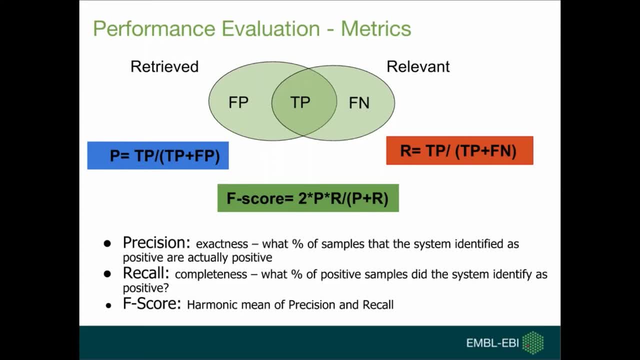 as well as the relevant ones. The text mining tool retrieves both relevant and irrelevant documents. The Venn diagram shows the overlapping documents between the retrieved set by the tool and the relevant set within the pool. The relevant documents which are missed by the tool are called as false negatives. 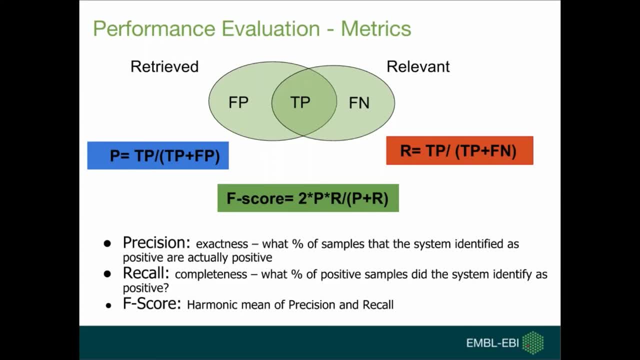 The relevant documents which are retrieved by the tool are called as false positives, And the relevant documents which are retrieved by the tool are called as true positives. False positives, false negatives and true positives are used to estimate the system performance in terms of precision, recall and F-score. 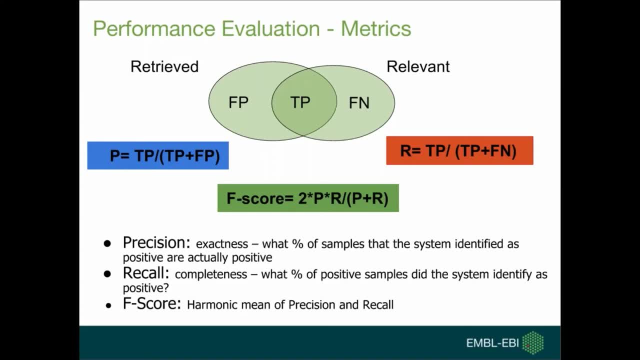 Precision presents the exactness of the system and measures the performance of the system. The Venn diagram shows the overlapping documents. The Venn diagram shows the overlapping documents. It measures the percentage of samples that the system identifies as positive or actually positive. It is calculated by the equation showing in blue. 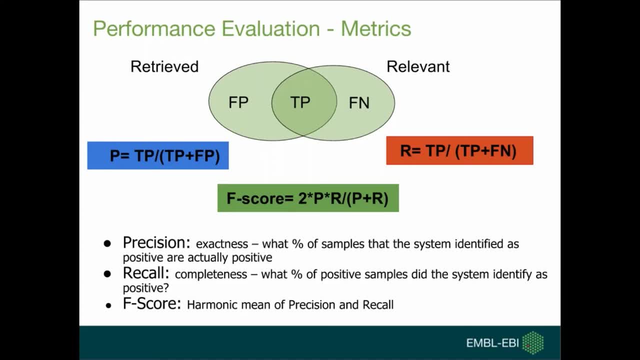 Recall presents the completeness of the system and measures the percentage of positive samples which the system identifies as positive. It is calculated by the equation showing in red. An FC-Core is the harmonic mean between precision and recall. It is calculated by the equation shown in green. 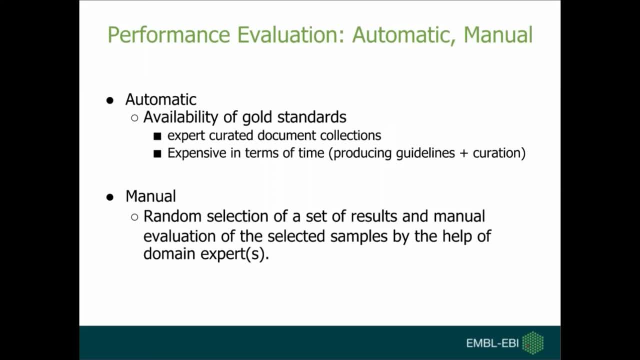 There are two ways to evaluate a text mining tool's performance. One is automatic and the other one is manual. Automatic evaluation is applied if there is a suitable gold standard corpus exists. Gold standards are expect greater data sets and it's very expensive to develop them. 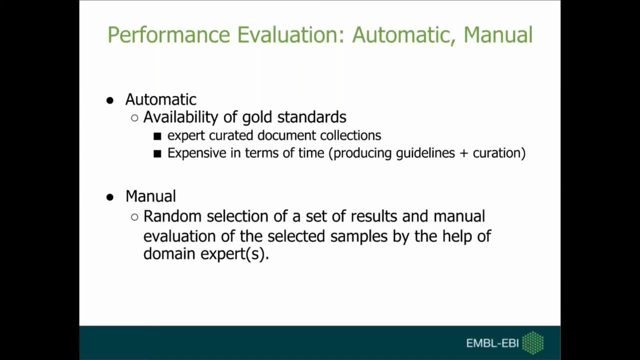 It requires certain amount of time to produce annotation guidelines and create the data. Therefore, there is no gold standard yet for many of the text mining tasks. Manual performance evaluation is applied in such cases, which involves random selection of a sample result set and hand creation by domain experts. 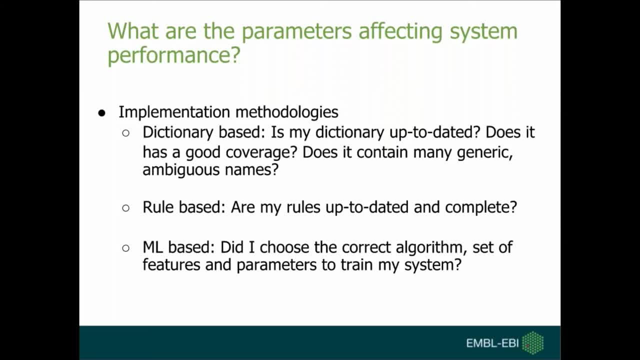 In order to design a good performing system for a dictionary-based approach, we should use a high coverage, up-to-date resource. Also, the quality of the entries in the resource should be considered. This resource should be screened for positive, generic or ambiguous entries, since such entries would cause to retrieve many false positive results. 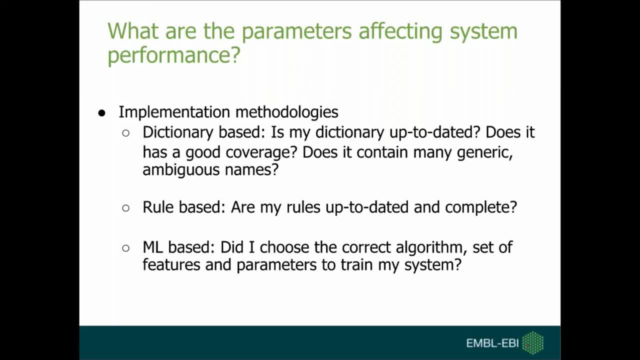 For a rule-based system, we should ensure that the generated rules are up-to-date and complete. For a rule-based system, we should ensure that the generated rules are up-to-date and complete. For a machine learning-based system, we should carefully choose a suitable learning algorithm among the many available ones, such as support vector machines and neural networks. 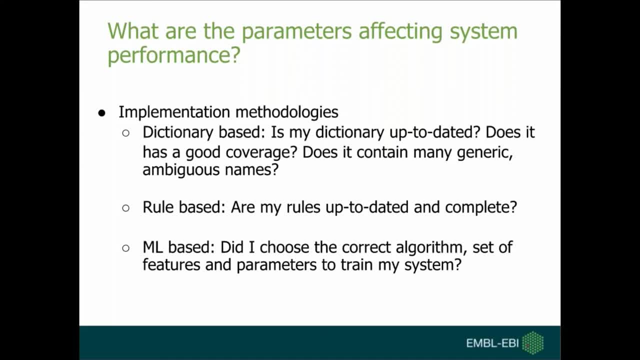 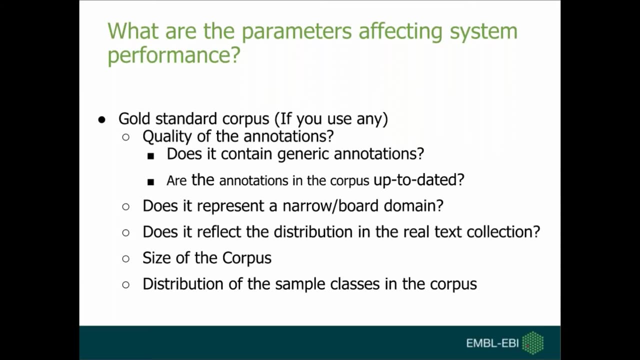 Feature selection and setting up training parameters also play a role in the system's performance. in machine learning-based systems, Another parameter affecting performance is the gold standard data set used. Another parameter affecting performance is the gold standard data set used. Another parameter affecting performance is the gold standard data set used. 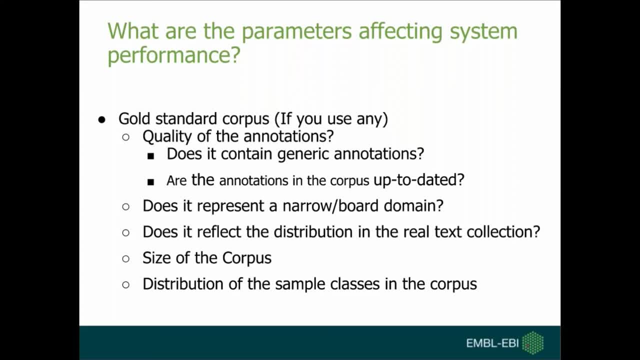 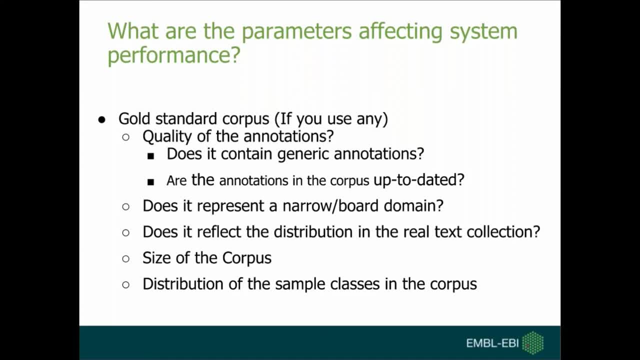 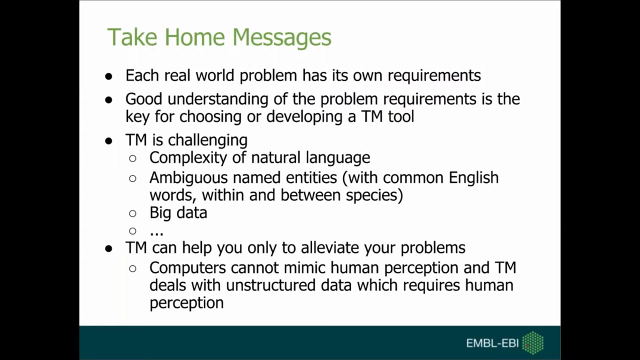 would have poor recall on the real text collection due to many missed samples. Similarly, if the gold standard presents a narrow topic, its size is small or contains some underrepresented sample classes, the system would achieve very poor performance in real settings. Let's close this session by providing some take-home. 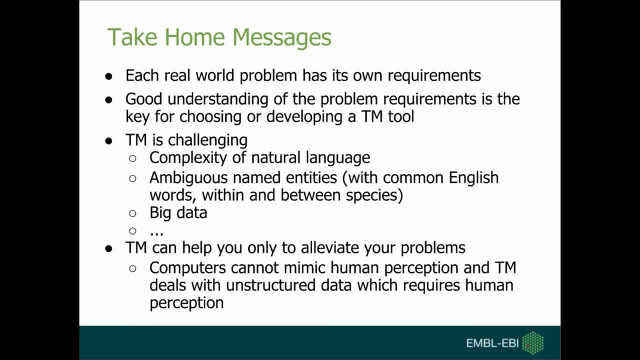 messages. Firstly, each real-world problem has its own requirements. Therefore, good understanding of the problem requirements is the key for choosing or developing a text mining tool. Text mining is not trivial. It is challenging due to many issues. Firstly, text mining deals with natural language. 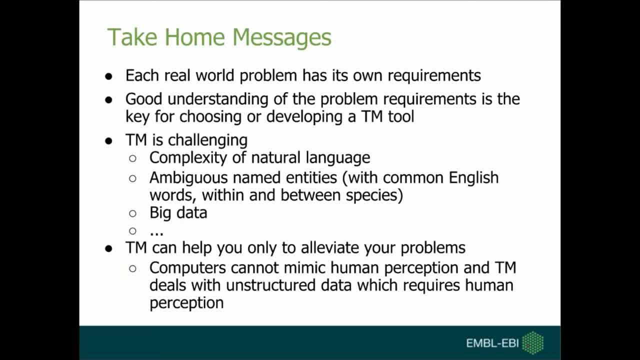 which is complex and unsubstantiated. This data is ambiguous, For example, name entities are ambiguous with common English. In addition, the literature has a massive volume, making text mining as a big data problem. Therefore, text mining can help us only to alleviate our problems. 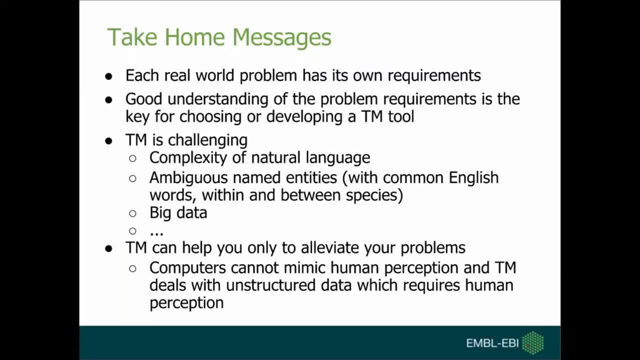 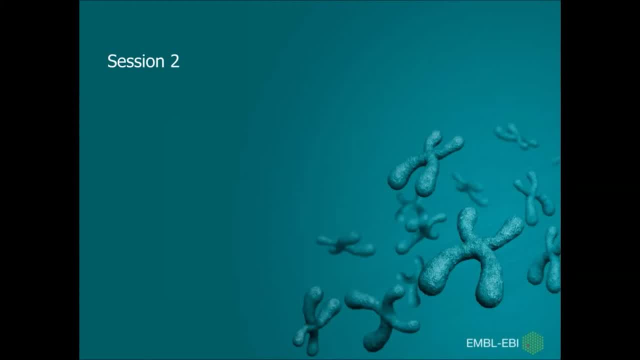 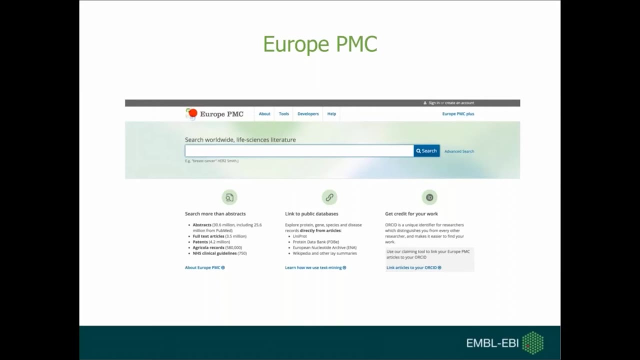 Computers cannot mimic human perception, and text mining deals with unsubstantiated data, which actually requires human perception. This is session two. In session two we will present European Med Central and how you can build your own pipeline. European Med Central is a search engine for biomedical literature. 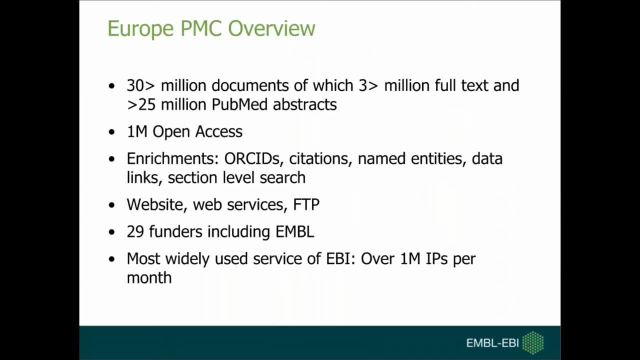 It contains over 30 million documents, of which 3 million full text and over 25 million PubMed abstracts. Among 3 million full text articles, one million is European Med Central is open access articles On Europa Med Central. we try to reach articles using: 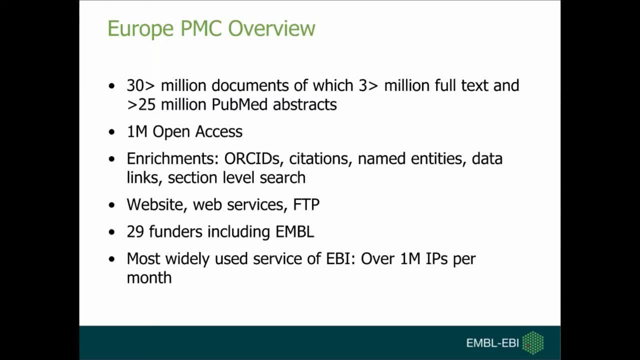 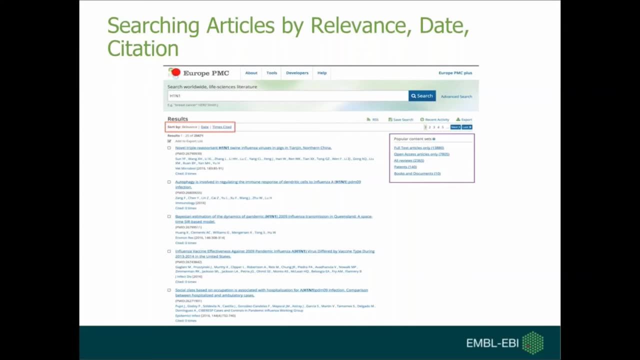 several ways. like we do citations, we identify named entities, we provide data links and also we do section-level searching. On Europa Med Central, there is only one search box for both redline abstracts and PubMed Central full-text articles. Search results can be ordered by relevance, date or the number of 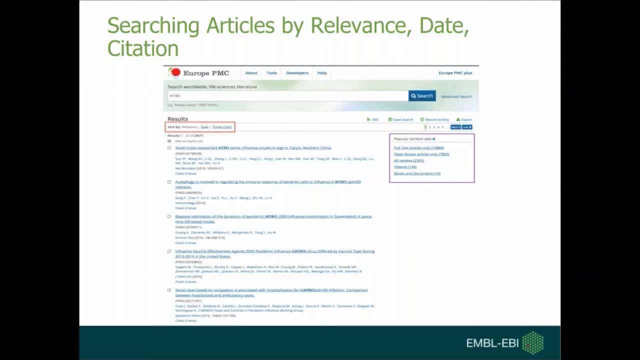 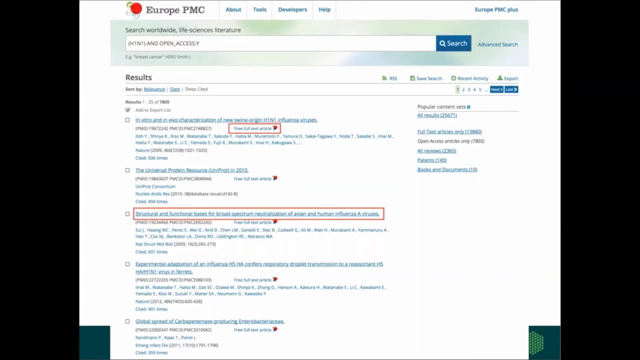 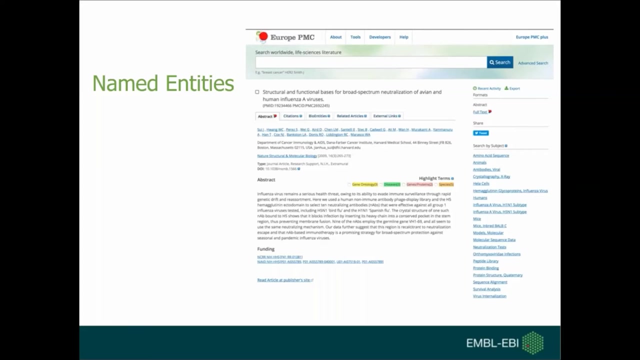 citations of that particular paper. On the list of retrieved documents you can see what are full-text articles. You can also select only open access articles. among full-text articles On Europa, Med Central, we mine named entities and you can see those results for each article. For example, if 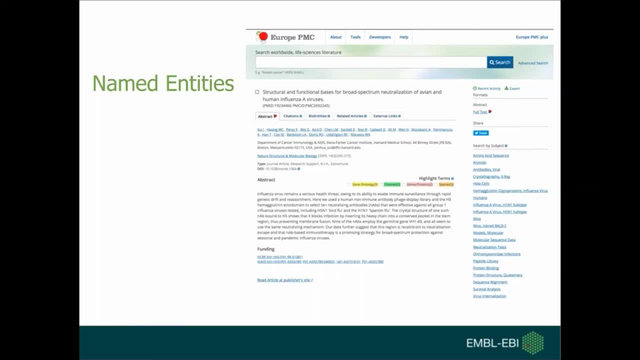 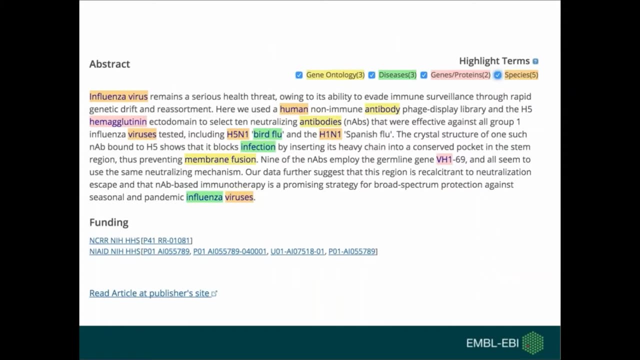 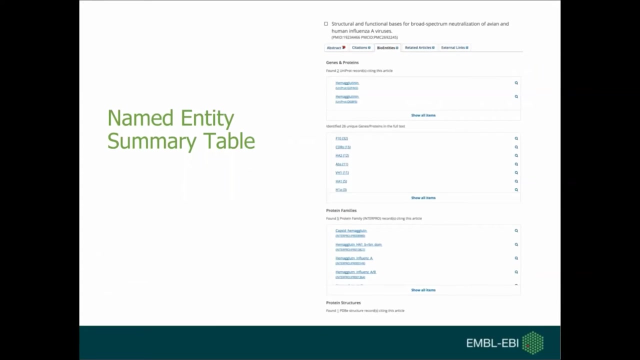 you visit an abstract, you will see those different colors on abstract. If you click those colors you will see all those named entities, For example disease names, gene, protein names and species. Another view of text-mined results, particularly for named: 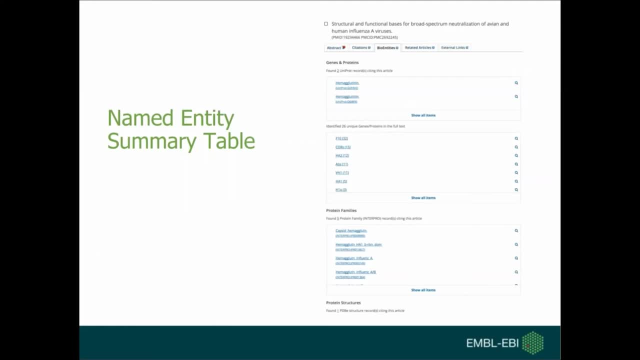 entity recognition is a summary table. You can have all those named entities mentioned in full-text articles in a tabular style so that you can, instead of reading the whole article, you can quickly go through what genes, disease names are mentioned, what GOAT terms are. 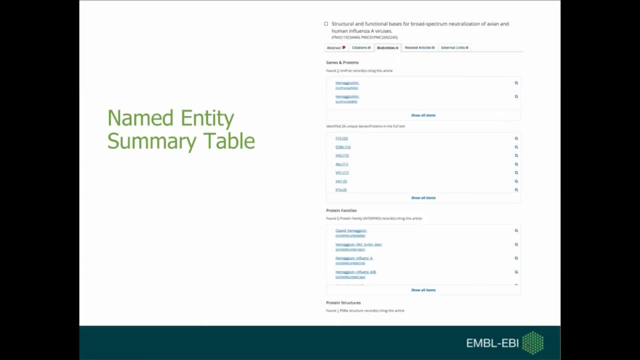 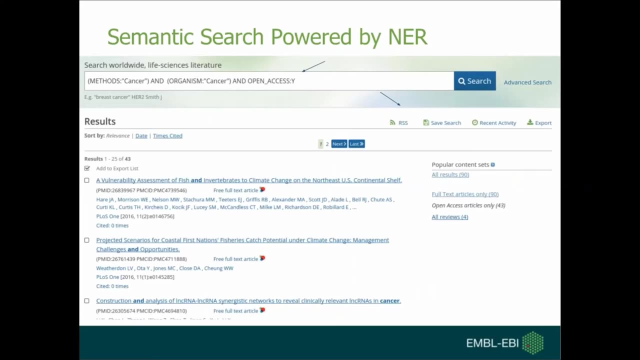 mentioned or what EFO terms are mentioned. quickly, Thanks to text mining, you can do semantic search on Europe MedCentral. This is the example I mentioned in introduction where, when you want to have all those articles where cancer is a genus and mentioned in section, You can write a Boolean query. 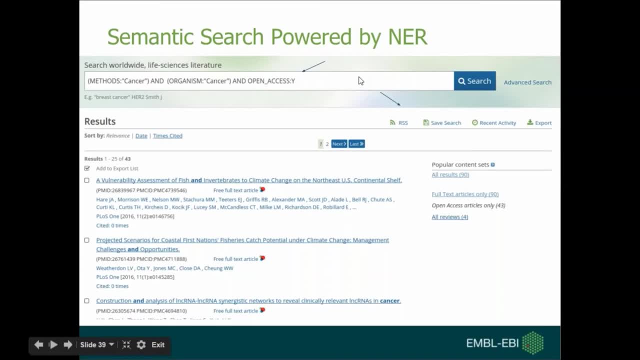 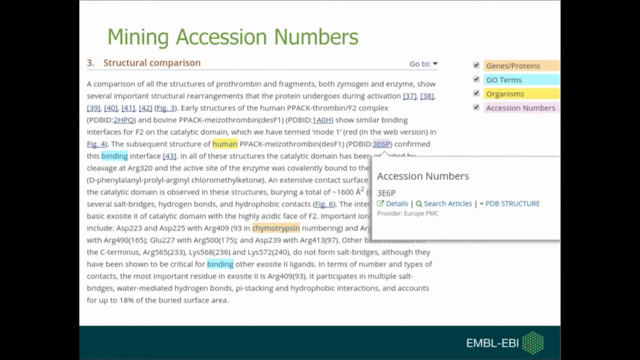 like this and this will give you those 90 rare articles, which is very important, related to your own query On Europe MedCentral. we also mine accession numbers for data citation. For example, in this article we identified PDB accession number and if you click the highlight, it will give you a box where 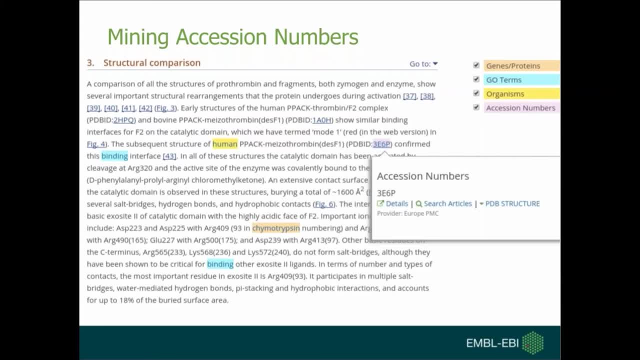 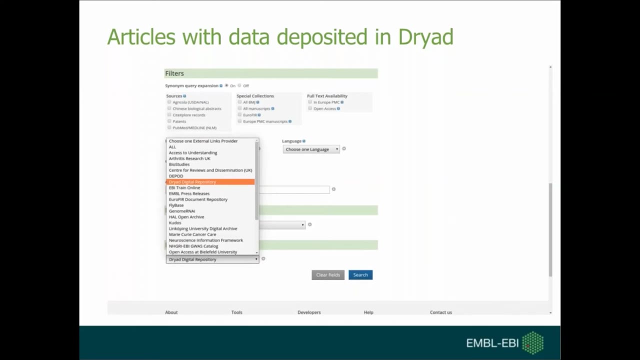 you can find more details on that particular accession number. For example, if you click PDB structure on this box, you will get the structure of this particular protein On Europe MedCentral there is a mechanism called external links by which user can provide relevant URLs to Europe MedCentral. For example, if you read the: 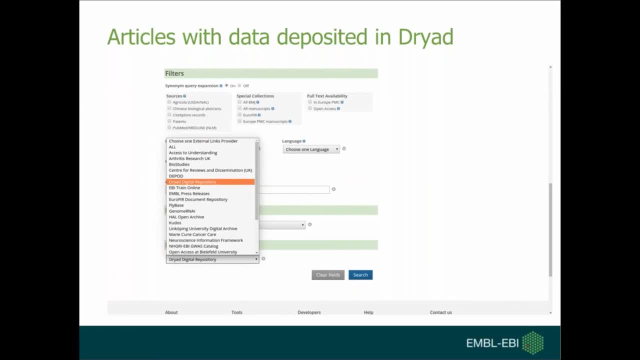 deposited data in Dryad and you know relevant articles. you can provide a mapping table between those data you read deposited and those articles related. That will make index built on Europe MedCentral and you can make search such as: can I get all those articles linked it to a particular data? 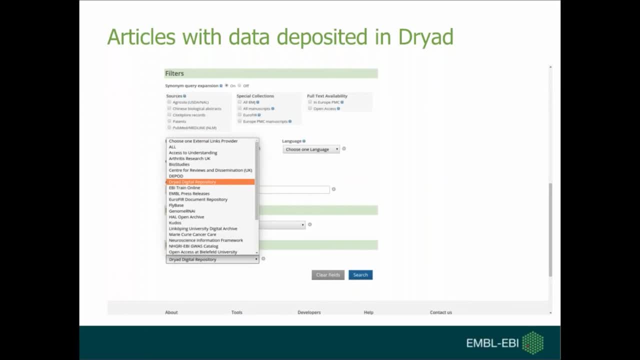 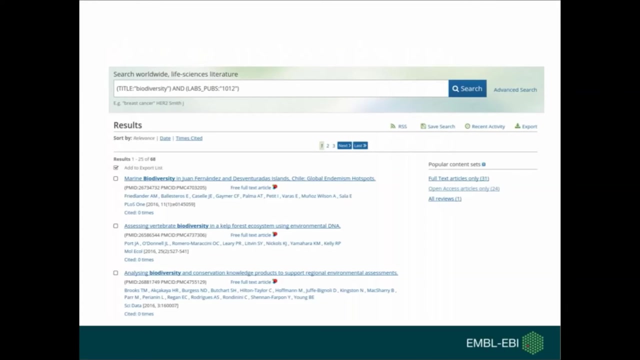 For example, on Europe PubMed Central advanced search setting, there is a section for external links where you can choose a particular data repository, in this case Dryad. Then you can make a query like: can I get all those articles where biodiversity mentioned? 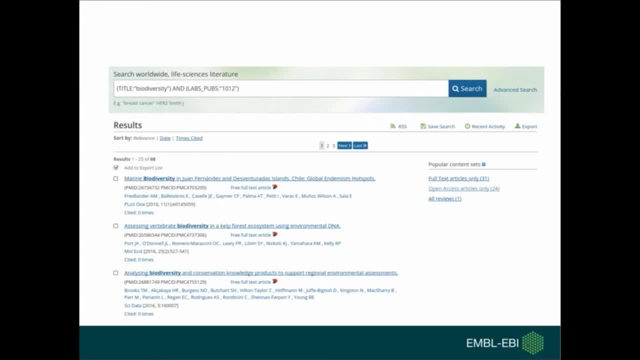 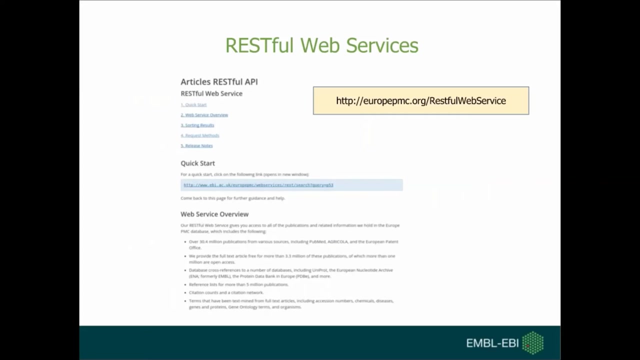 in title and also those articles linked to data in Dryad. This query will give you all those articles. Europe PubMed Central also provides RESTful web services- All those features I mentioned in the previous slides. you can also use RESTful web services. 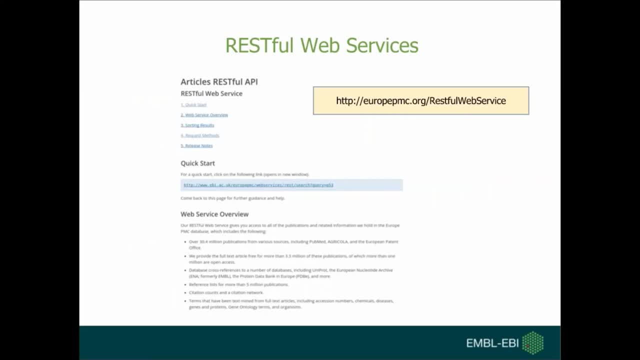 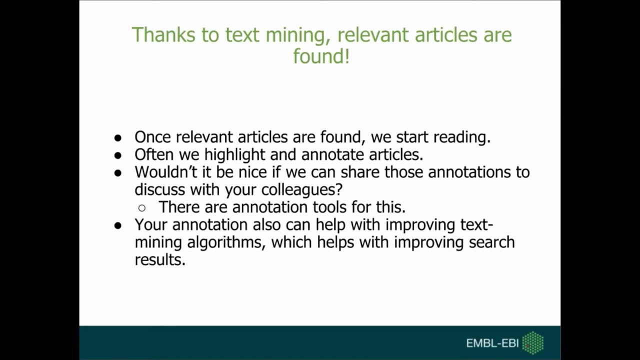 in order to get the same features. This is the URL for the RESTful web services on Europe PubMed Central. If you want to know more details, please visit this URL. Next to Text mining: now you have relevant articles found. Once articles are found, you are going to start reading. 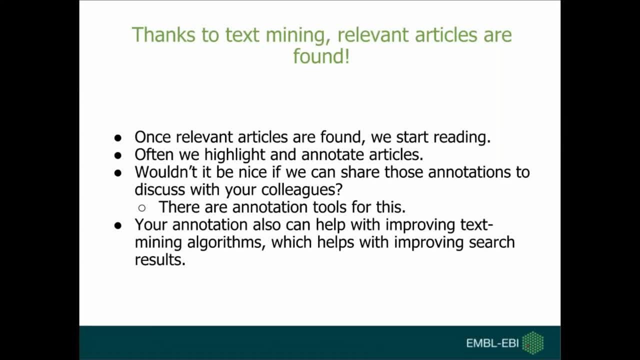 While you are reading, often you are going to highlight and annotate those articles. Wouldn't it be nice if you can share those annotations and to discuss with your colleagues? There are annotation tools for this. Your annotation also can help with improving text mining algorithms, which will 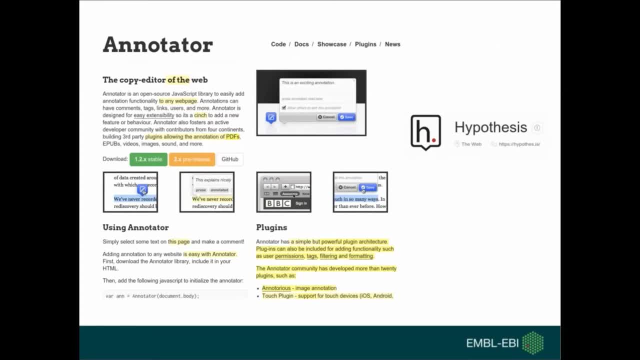 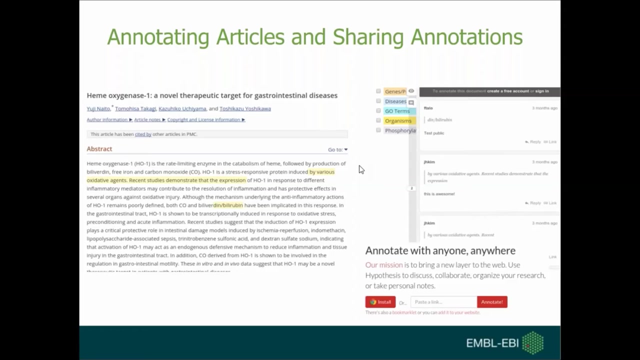 help with improving search results. Annotator is an open-source JavaScript library for annotating web pages On the top of Annotator. Hypothesis provides annotation platform. This is an example of annotating an article with Hypothesis on Europe and MedCentral. You can see the highlighted part, which is commented by: 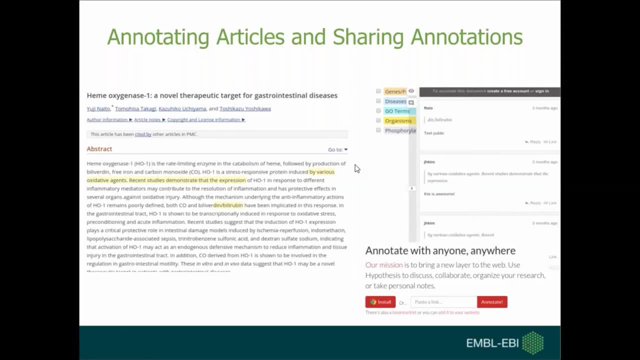 a user and this is shared And you can see other users also commented on that particular part. As I said, using Hypothesis like annotation tool, you can annotate your article and you can share those annotations with your colleagues In order to use. 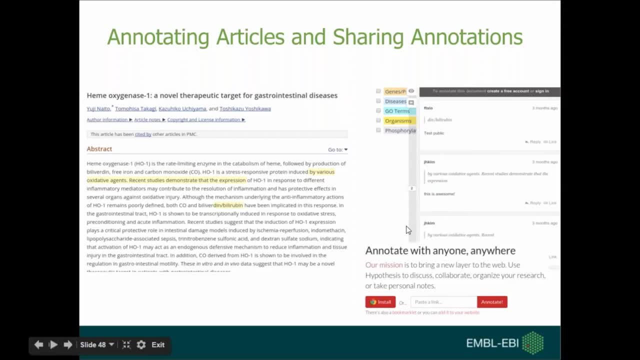 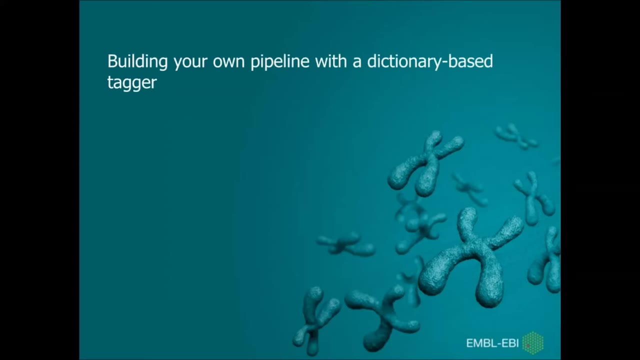 Hypothesis: you just need to install a plugin for major browsers. You just go to website and you can download and you can install those plugins into your browser. Sometimes, tools available for text mining is not good enough for your problems. In that case, you have to. 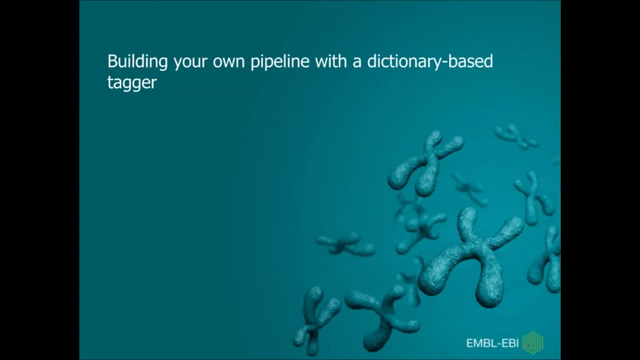 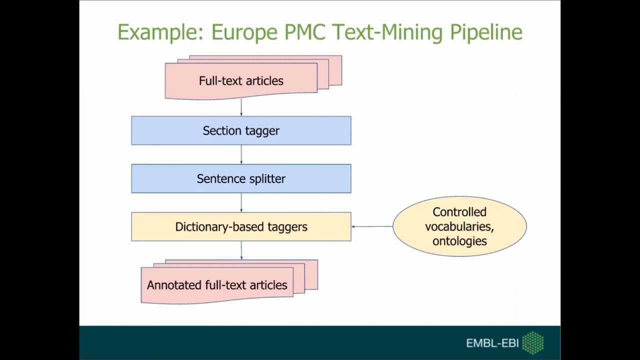 develop your own pipeline. In this part we're going to explain how to build your own pipeline. On this slide you can see our Europe and MedCentral text mining pipeline. This pipeline takes full text articles as input and the pipeline transforms those articles by several modules. First section: tagger Section. 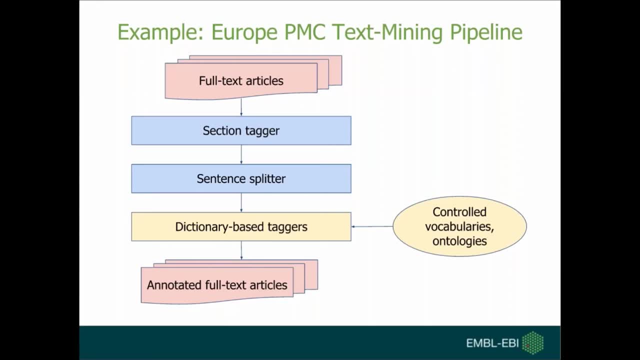 tagger identify different parts of articles into a list of sections, like introduction, method, result, discussion tables, figures, etc. Once you identify sections, then sentence splitter will be applied, which identifies sentences in each section. Once we identify sentences, we will apply dictionary-based taggers, which is the most 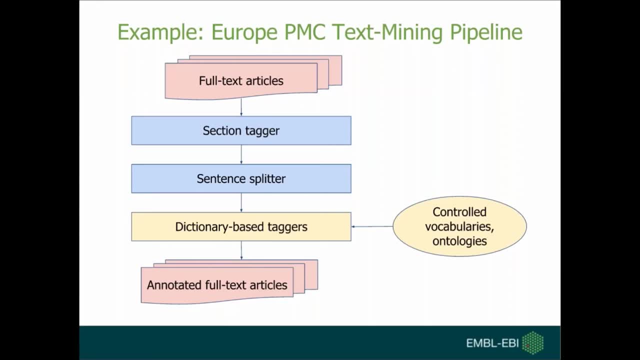 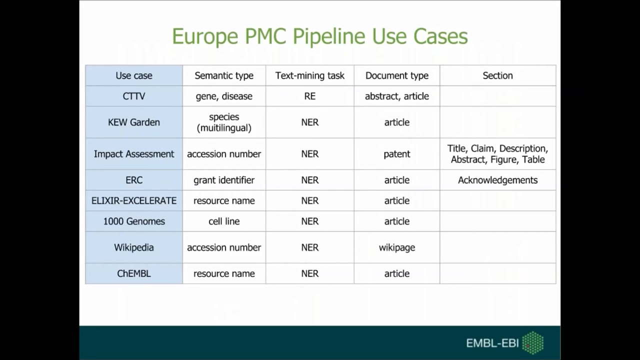 important part in pipeline. This is the key part for named entity recognition. After dictionary-based taggers applied, you will have automatically annotated full-text articles. Our Europermed Central text. mining pipeline has been also used for several use cases, mainly for mining. 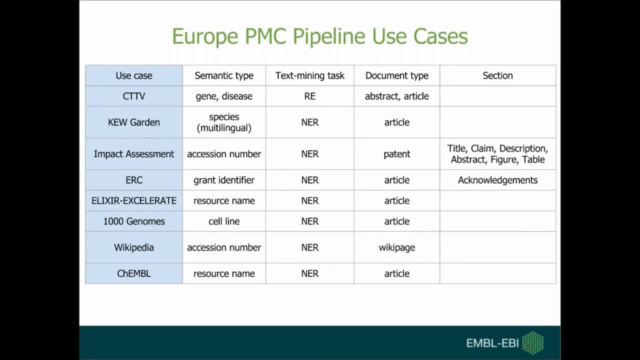 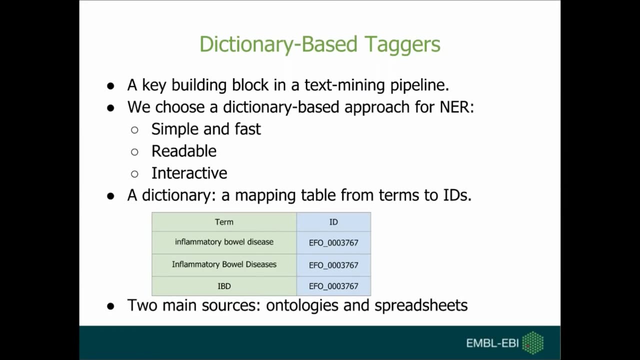 The pipeline has been also adapted for CTTV project in order to extract relations. Dictionary-based taggers are a key building block in our text mining pipeline. We have chosen a dictionary-based approach for named entity recognition because this approach is simple, fast and easy. 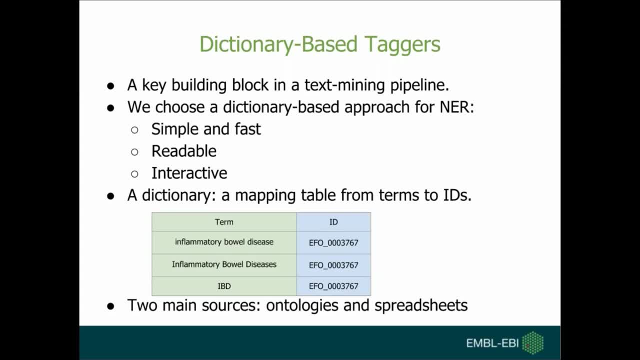 It is easy, fast, readable and interactive with domain experts like you biologists. What is dictionary Dictionary is a just mapping table from TOMS to IDIS, as you can see in this table, For example, the disease: inflammatory bowel disease. 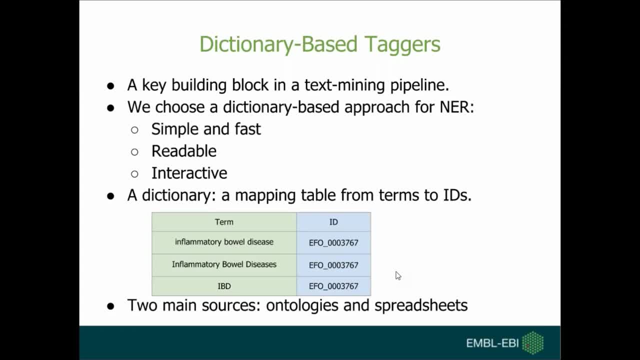 Dictionary-based taggers. The national hours of death has been mapped to the particular year for ID 003767. in this case, We call it this as concept. The same concept can be represented in different terms, For example here like IBD, which is abbreviation of coarse region. 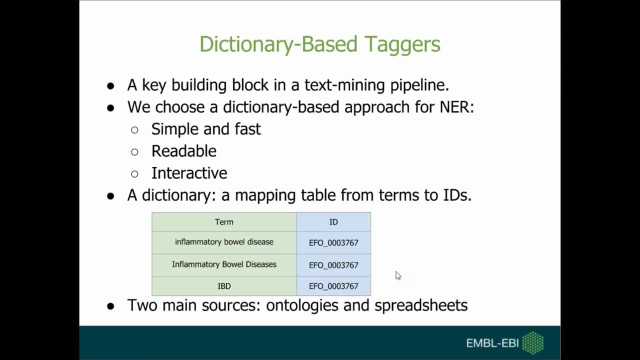 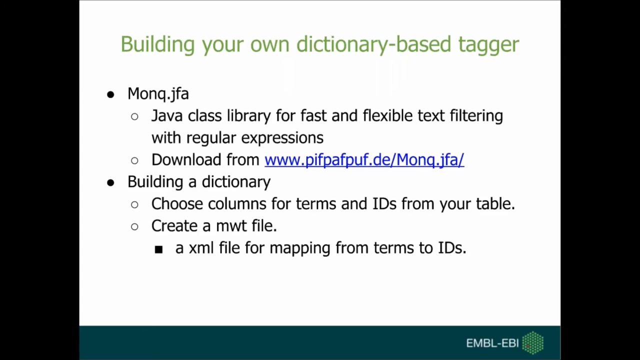 The brigonette device has a newly announced article using the loginch ap s, the disease name. This will be also mapped to the same particular ID. In order to build dictionaries, there are mainly two resources: ontologies and your own spreadsheets- In order to build a dictionary-based tagger. here we will use Monk JFA, which is 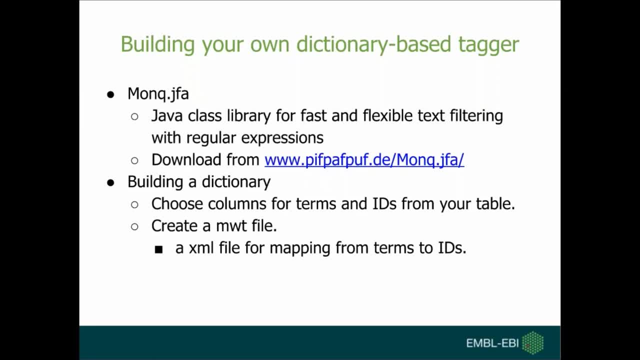 a Java class library for fast and flexible text filtering with regular expressions. You can download this program from the following URL. In order to build a dictionary, first you have to choose from your table what should be your tagger, The terms and what should be the IDs. Once you choose the right columns for terms and 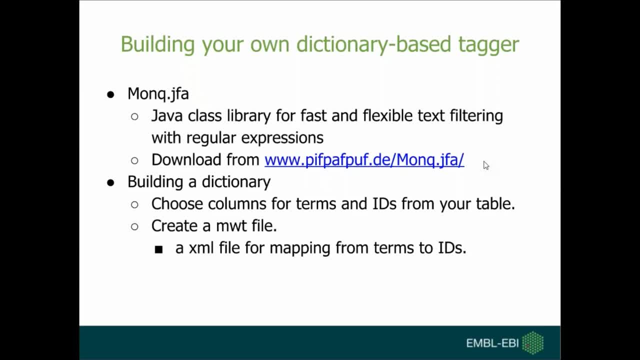 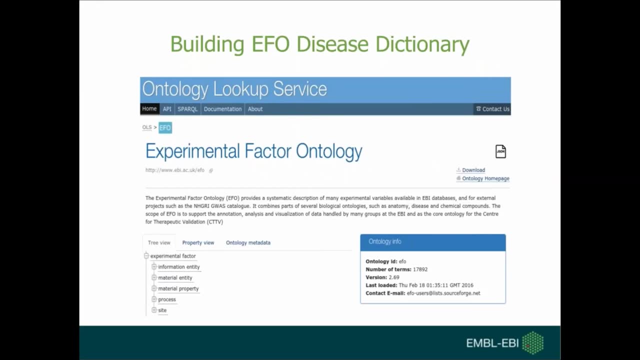 IDs, then you need to create MWT file, which is just XML file for mapping from terms to IDs. For this presentation, we will build EF4DiseaseDictionaries. First you can go to Online Lookup Service developed by EBI where you can find the right. 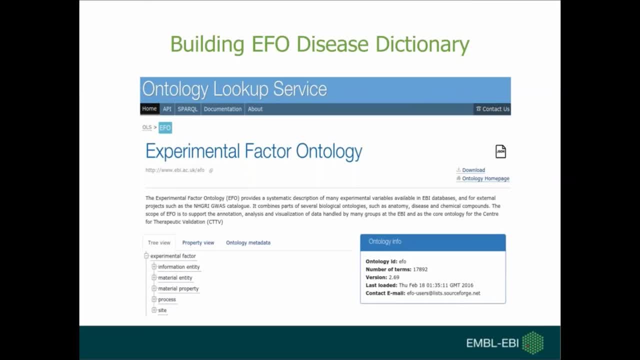 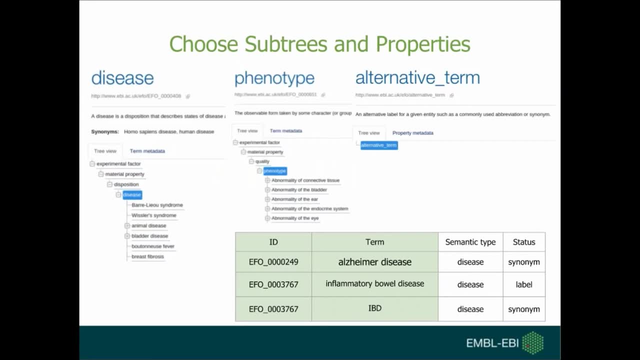 ontology for you, In this case, Experimental Vector Ontology. Once you choose your own ontology, the next step is you need to choose a tagger for each of the two products. The tagger will be the one that you are referring to. 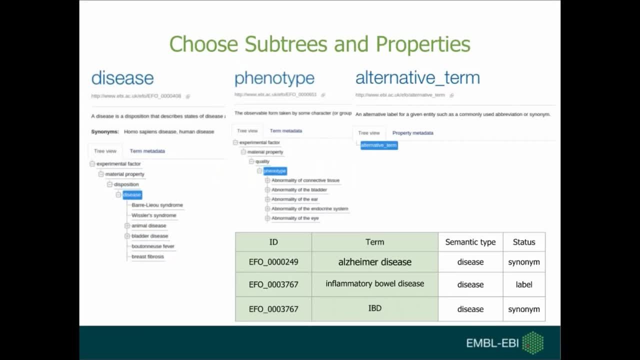 You can then just click on it and enter its name and date or date tagger And once you are subtrees of that ontology To build EFO disease ontology. we have chosen disease subtree and phenotype subtree. You also need to choose properties, which you can. 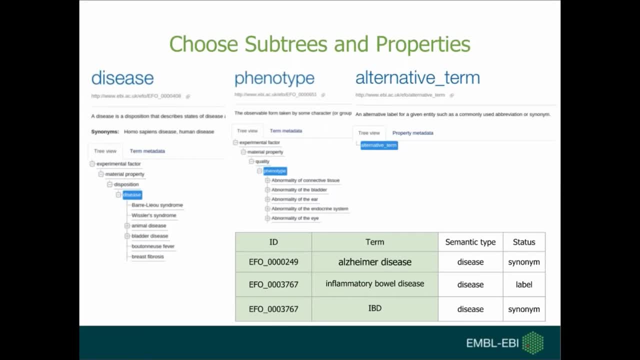 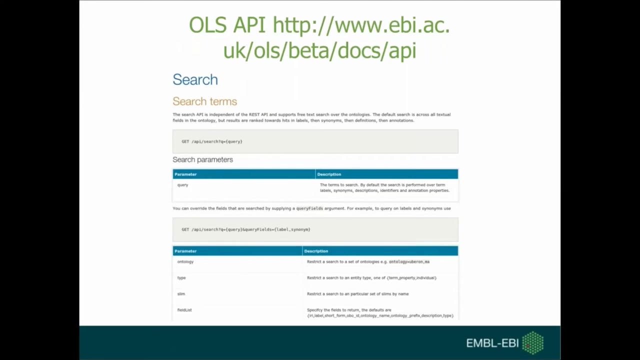 use for selecting terms in your dictionary. One example of the table we generated by choosing those subtrees and properties And in order to build a dictionary, we used only two columns, which are ID and tongue. In order to get this table, you can use the API provided by OLS and, if you need, 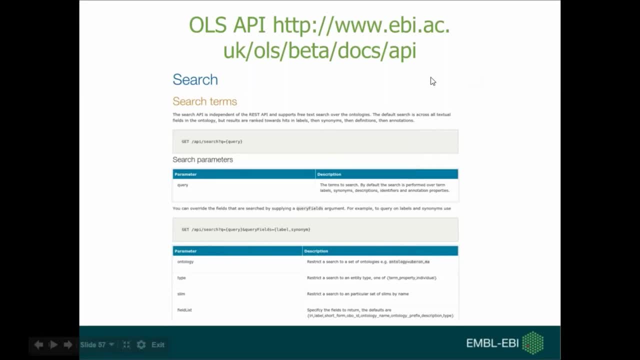 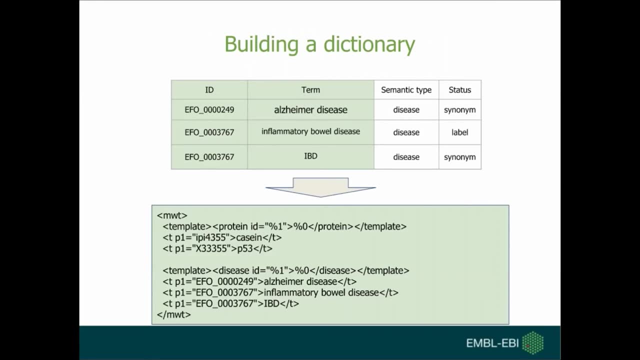 more details, please visit the URL mentioned here. Once you have a table and once you choose the relevant columns for your dictionary, now it's time to create a table. The table is now available on the local website. It's also in the create a MWT file. This is just an XML file where you can specify those mappings from. 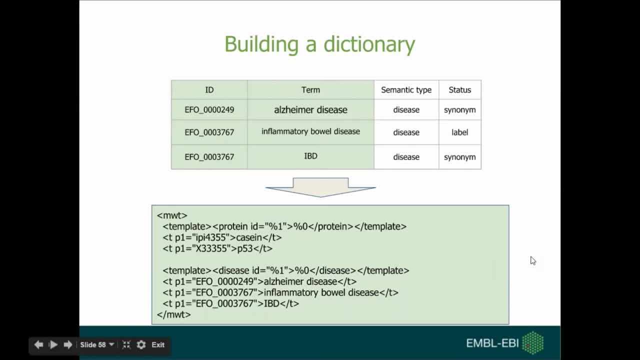 TOMS and IDIS. In this file there are two key elements. One is template and the other is TELEMENT. TEMPLATE describes the output to be produced on a match and TEA describes a dictionary TOMS you are using to build your dictionary From this table. we need to write: 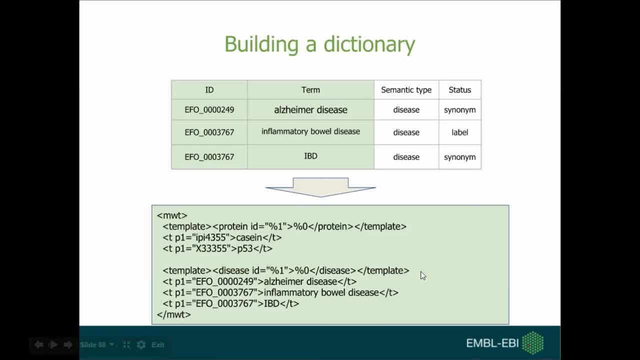 the following lines where we specify what the output is going to look like. This line means: whenever you identify something that will be marked as disease. These are the list of TOMS from this table. For example, we put Alzheimer's disease with the corresponding EF4 ID. We did the same for inflammatory bowel disease and IBD, with different. 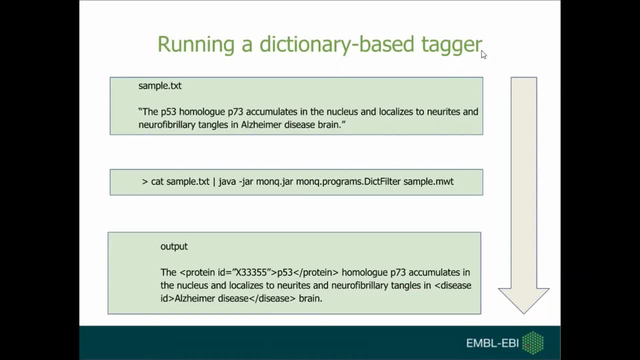 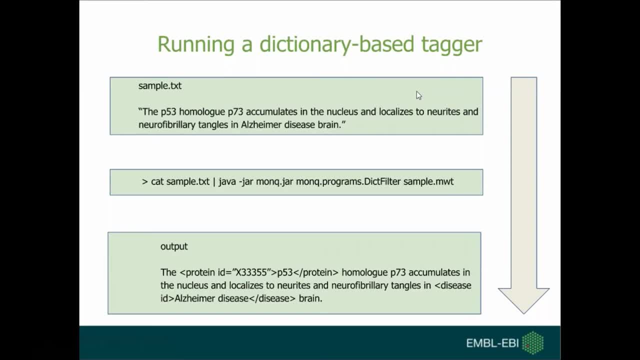 example, and this is the first example Here I put one sentence in the file SAMPLEtxt. Here I put one sentence in the file SAMPLEtxt: On Linux machine you can run your tagger to that particular sample file. This is the. 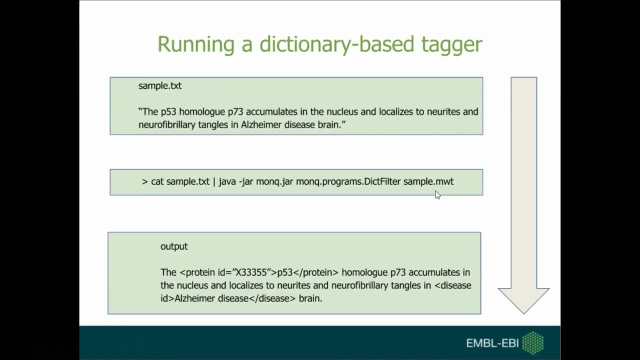 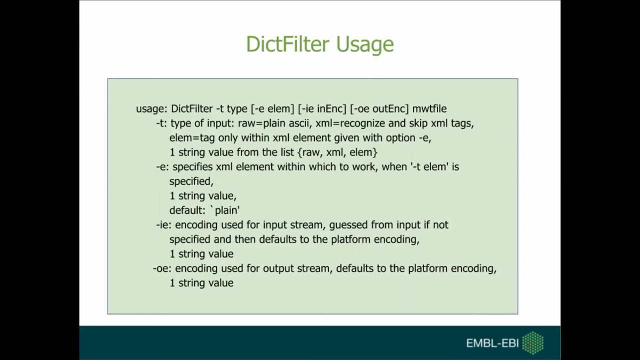 Java command you can use once you download the MONC jar library and once you have your own dictionary. After running your tagger, you will get an output where gene, protein names and design names are identified and marked using XML elements. If you want to know more details, this program has a help page which you can refer to. 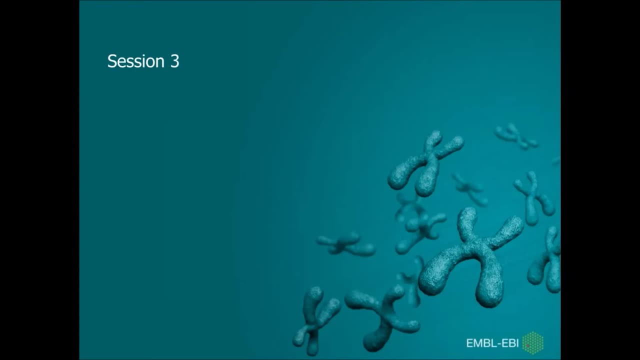 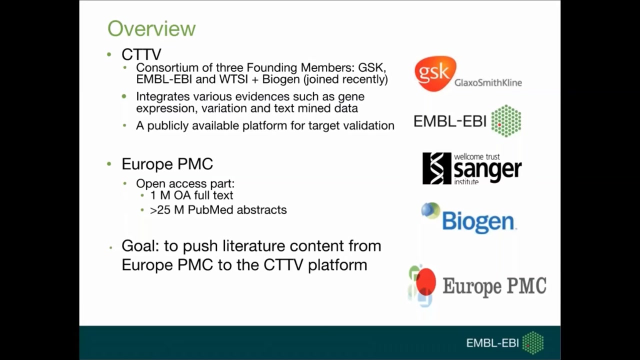 Session 3.. In this part, I will provide you an industrial project as a sample text: mining application. CTTV stands for Center for Therapeutic Target Validation and it is a consortium of three founding members, Including GSK, which is a pharma company, EMBL-EBI and Wellcome Transanga Institute. 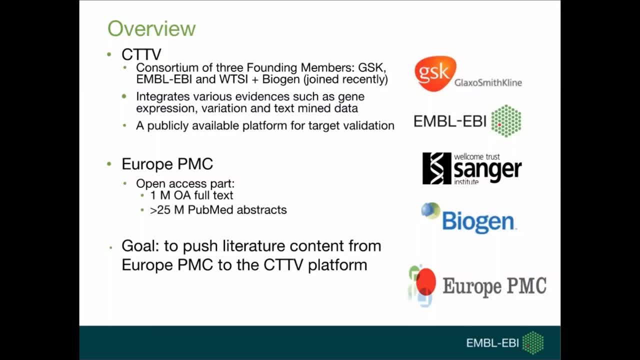 And recently, another company called Biogen has recently joined them. The aim of CTTV is to integrate evidences from various resources, such as gene expression and variation data, and also text mining data, And provide a public access to the data. 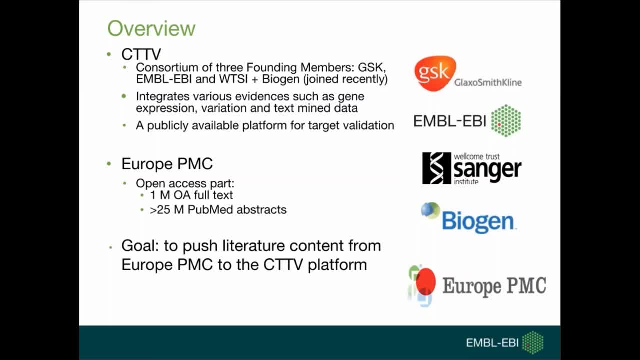 The goal is to create an accessible platform for target validation. In our text mining project, we use EuroPMC as the literature repository And extract only the open access parts of EuroPMC Because, due to the licensing agreements, we can text mine only open access part. 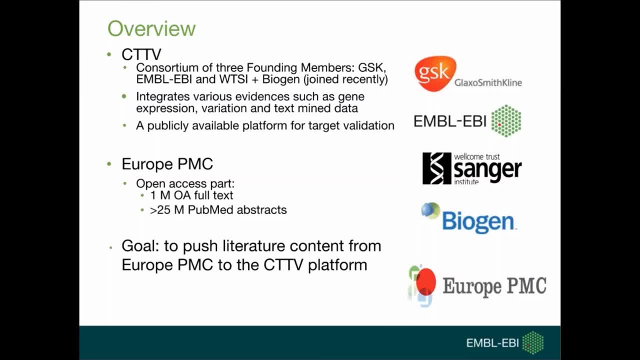 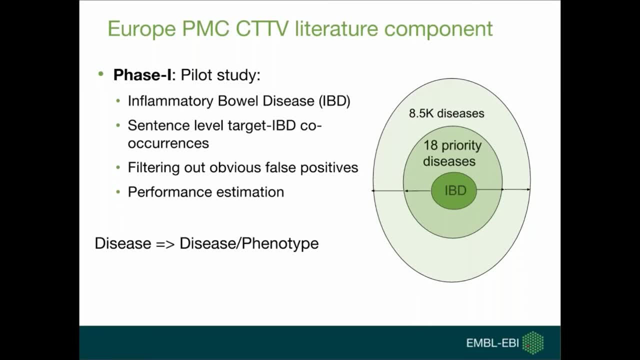 And extract gene disease relations from articles And submit this data to the platform. Our project consisted of three phases. Phase one, called pilot study. In the pilot study we focused on a single disease, which was inflammatory bowel disease, And extracted gene disease co-occurrences at the sentence level. 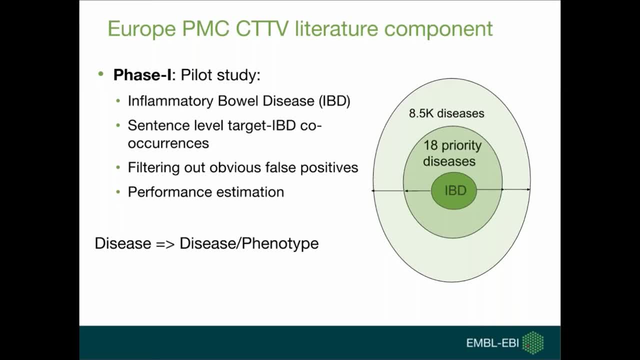 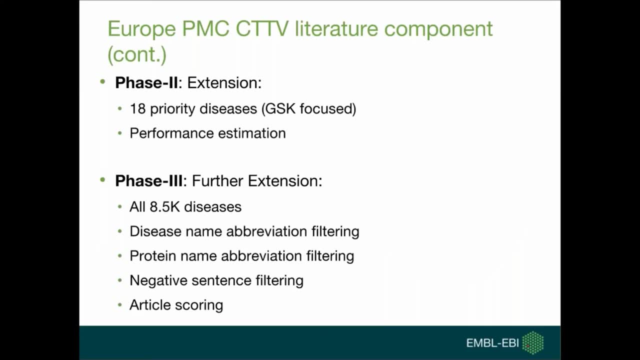 We filter out obvious false positive and estimated the performance. Session 4. Session 5. Session 6. Session 7. Session 8. Session 9. And in the second phase we extended the study to 18 diseases identified as priority diseases. 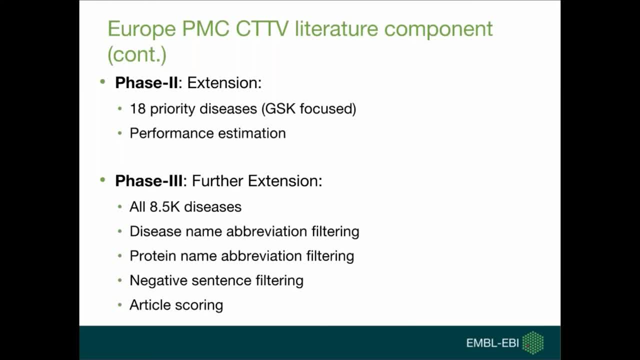 by GSK And we re-estimated performance to be sure that the system performance is stable. In phase three we further extended the study to all 8.5K diseases from EFO. We develop and use disease name abbreviations- Protein name abbreviations filter. 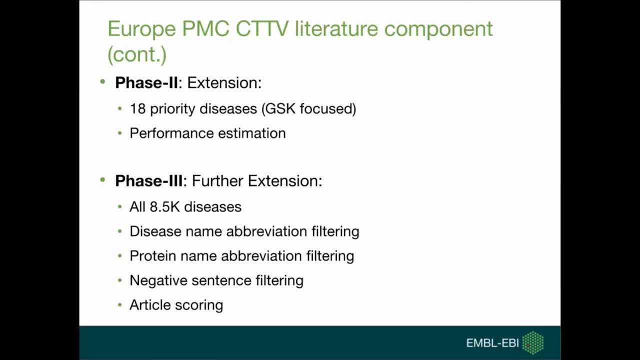 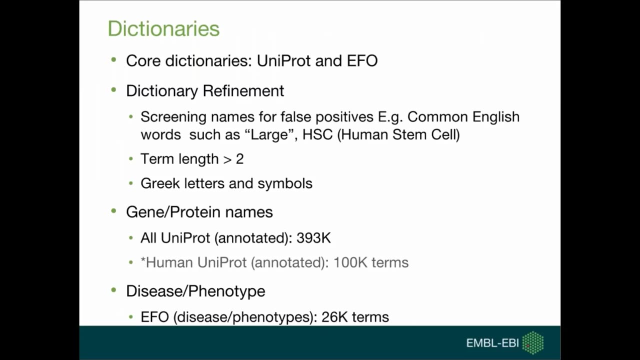 To filter out false positives from our results. We also used negative sentence filtering And we introduced article scoring. There are two core dictionaries used in this project. One of them is Uniprot, for identifying genes in text, And another one is EFO- experimental factor ontology- for identifying genes. 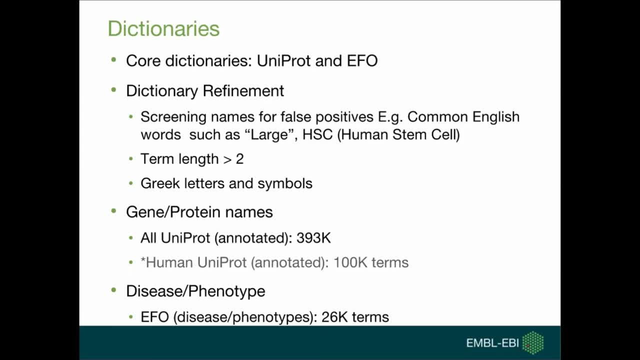 And the third one, EFO- For identifying the genes, in text. And the third one, EFO- For identifying gene type, And the third one, EFO. And the fourth one, EFO- diseases or phenotypes- in text. However, we applied some refinements before using the. 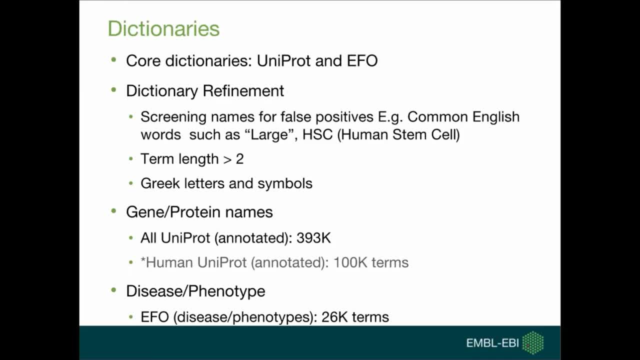 dictionaries. We screened dictionary entities for possible false positive terms. For example, some of the entries are ambiguous with common English words like large or other domain specific terms like human stem cells. We screened out all the ambiguous terms and we also screened out all the terms having length less than two, because such terms would introduce false positives. 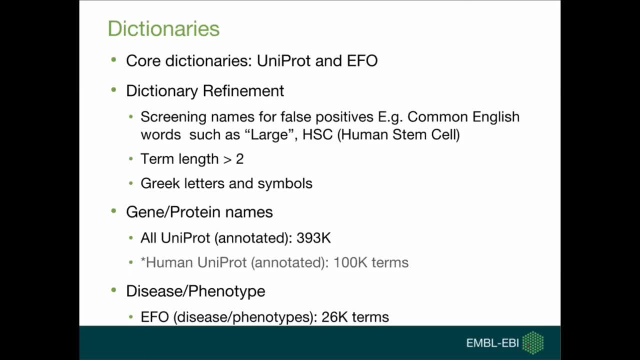 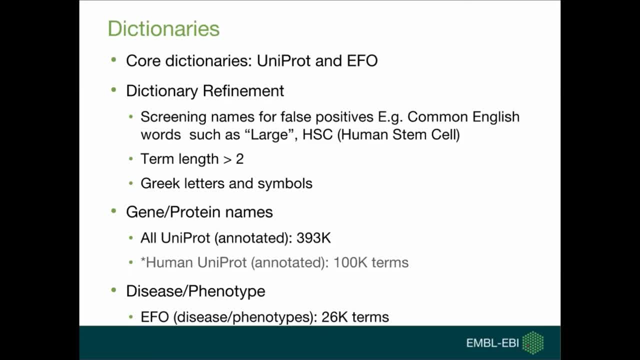 We use polygons to identify genes. We use polygons to identify genes. We use polygons to identify genes. So we actually saved the patient's sweeter about 60% of the time by using these 2 dictionaries: First health uniprot and the cityices dictionary is around 400 K, and later we used 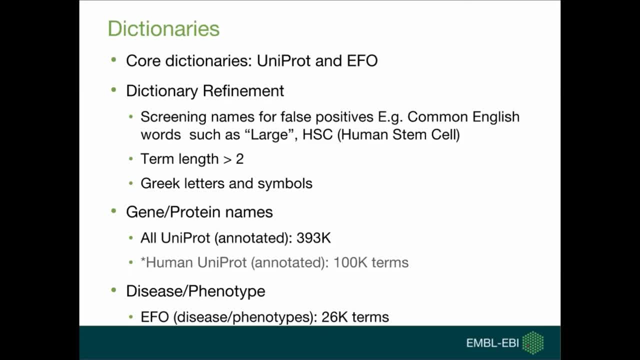 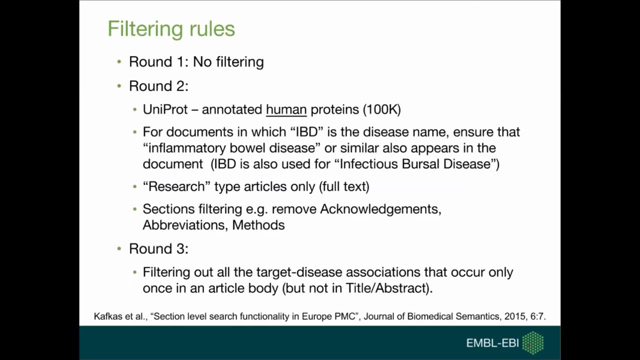 on the human part of Antep anschafi patit. Our disease dictionary size is 26 K. We applied filtering rules in three rounds. In the first round we didn't deline any filtering. In the second round we used only human part of Uniprot because we 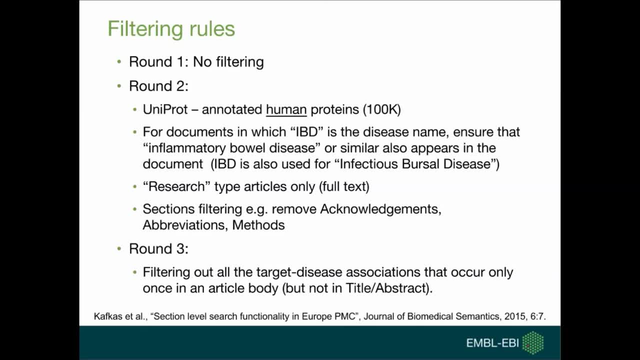 realized that using whole Uniprot would introduce us lots of false positive and we also ensured that the long form of a given disease name exists in the text in case the abbreviation of the disease name appears in text. We also focus in on the research type of articles, since other type of article like review, 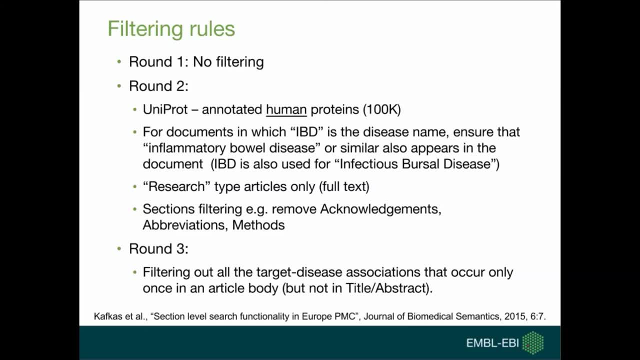 article would introduce false positives. We also screen articles according to section. We filter out some sections, For example acknowledgement, abbreviation, and probably would introduce false positives. achtmals jacks or extra Embasos. In this case we added time제 according to. 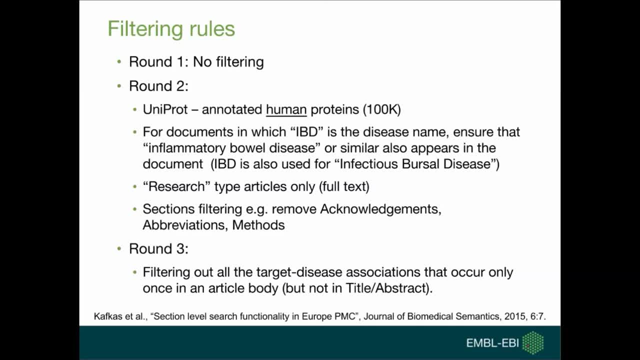 Countrys, so the nucleic acid examples also includedulate. 41% of instances is offered due to the fact that they would introduce false positives positives to the results. In the third round we filtered out all the target disease associations that occur only once in an article body but not in. 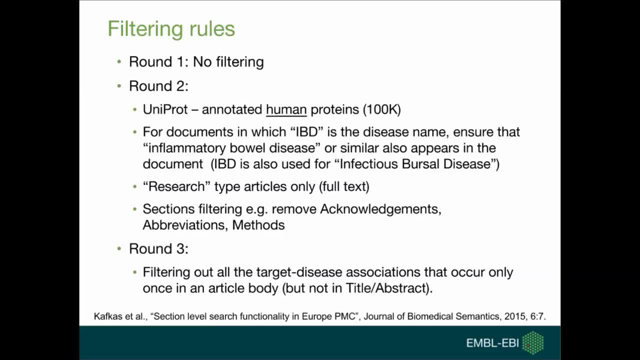 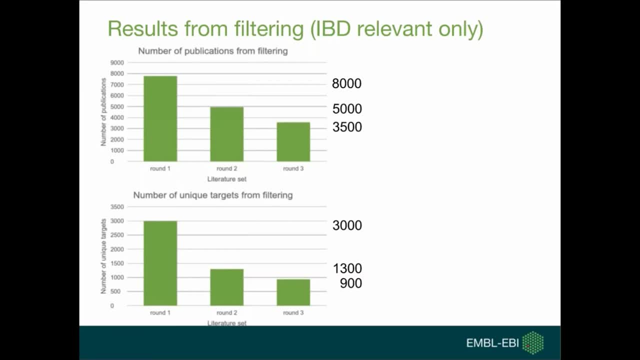 article title or abstract, because concurrences in article title or abstract would be the most confident concurrences. This graph shows the results from our filtering. In the first graph you see that we reduced the number of publications from 8000 to around 3500 articles, And in the second graph you can. 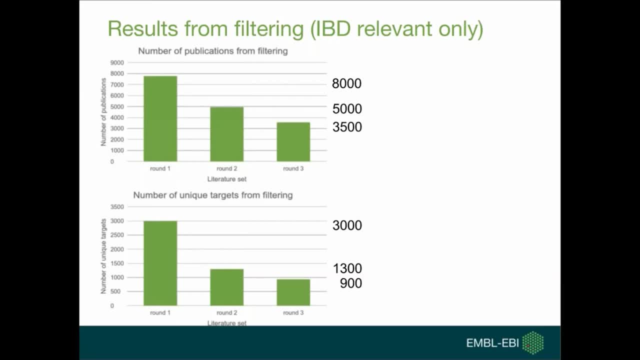 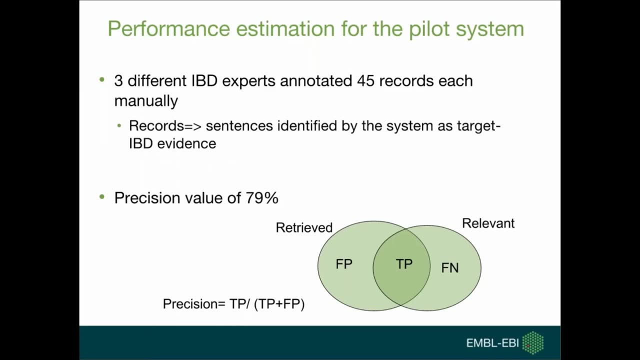 see that we managed to reduce the number of targets from 3000 to around 900.. We estimated the system pattern performance manually. For this purpose, three different IBD experts annotated randomly selected 45 records manually And the precision of the system was estimated as 97%. 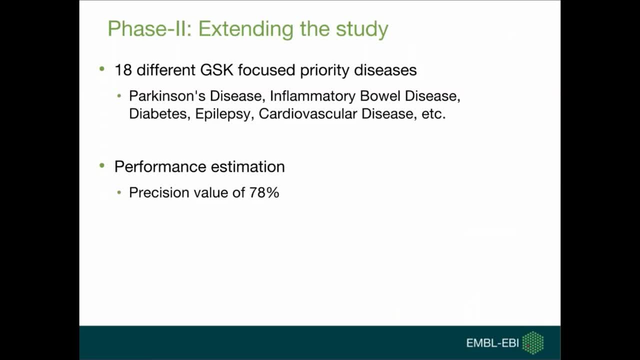 In the second phase we extended the study to 18 different GSK-focused priority diseases. Some of those diseases are Parkinson's disease, inflammatory bowel disease, diabetes, epilepsy and cardiovascular diseases. We re-estimated the performance to be sure that the system is still stable. 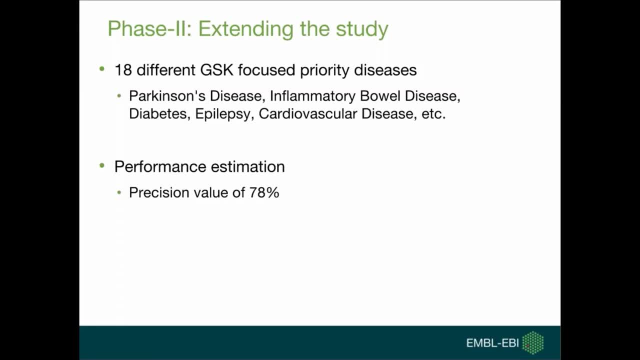 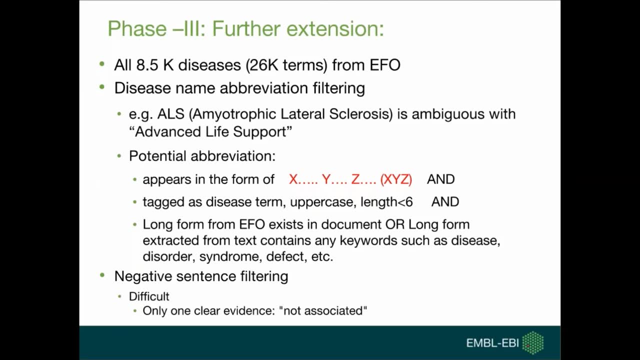 And the precision was estimated as 78%. In the third phase we further extended the study To all 8,500 K diseases from EFO. In this phase we introduced disease name abbreviation filter. Some disease names, for example ALS means amyotrophic lateral sclerosis- is ambiguous. 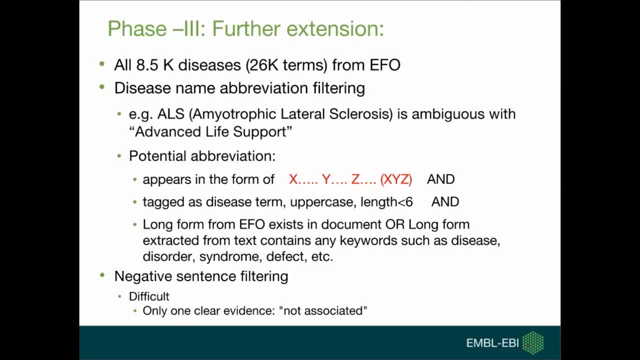 with advanced life support in some of the articles And you wouldn't like to annotate advanced life support In order to identify potential abbreviations in text. we use regular expressions and check for the text sequences showing in red. We call this the former part. 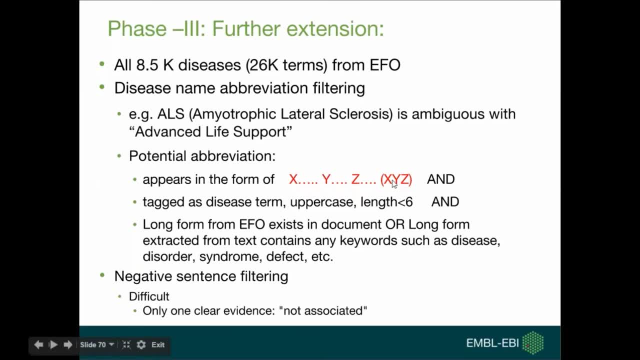 And we call this as potential abbreviation if it is tagged as a disease term by our dictionary, If it's in the uppercase, If it's in the lower case And it has length less than six, And we check whether the long form of the abbreviation from EFO exists in the document. 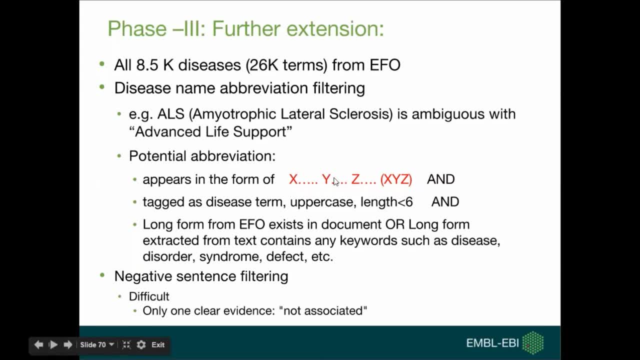 Or if the long form contains any of the keywords that were selected by our experts And for examples, These keywords are: disease, disorder, syndrome, defect. In this phase, we also filter out the sentences mentioning on negative associations. Due to the complexity of natural language, it is difficult to develop such a filter. 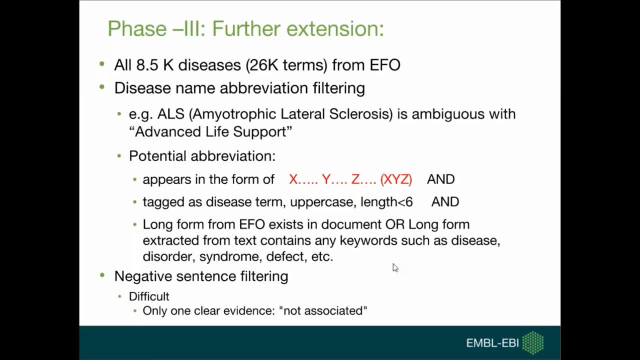 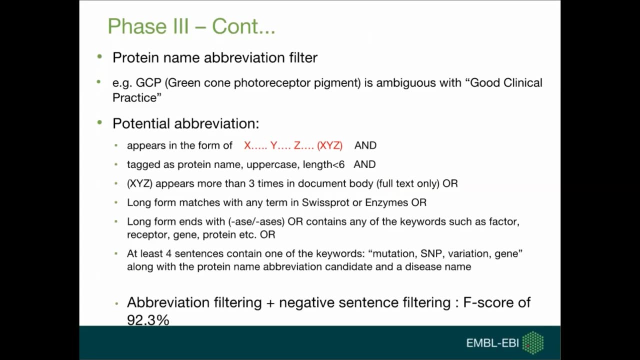 And the only clear evidence for us was the keyword not associated. So this is the only clear evidence for us: If a sentence contains not associated, it's filtered out automatically. We also introduce protein name abbreviation filter in phase three. Some of the protein names are ambiguous. 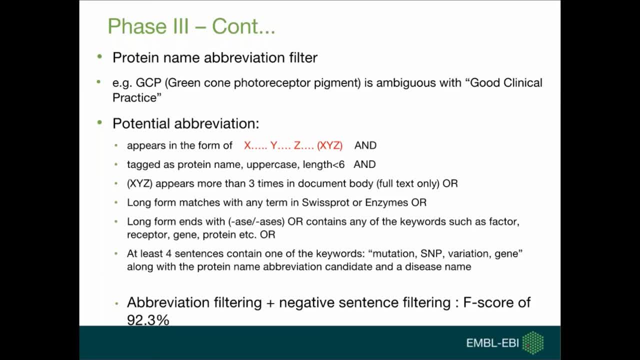 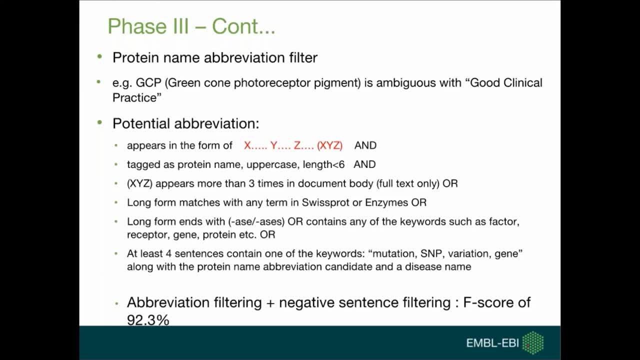 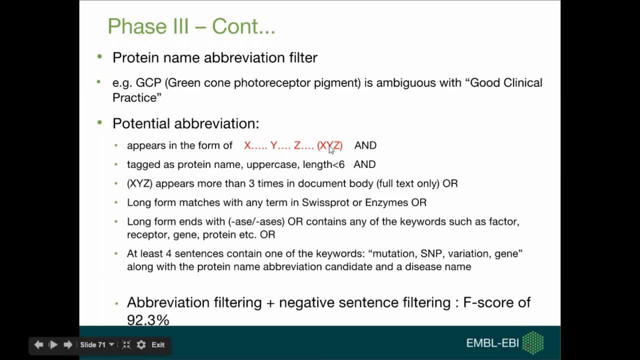 And the part appearing within parentheses as potential abbreviation. If it is stuck as a protein name by our target. If it is in the upper case form. If it has characteristics. If it has character less than six. We check whether the potential abbreviation appears more than three times in document. 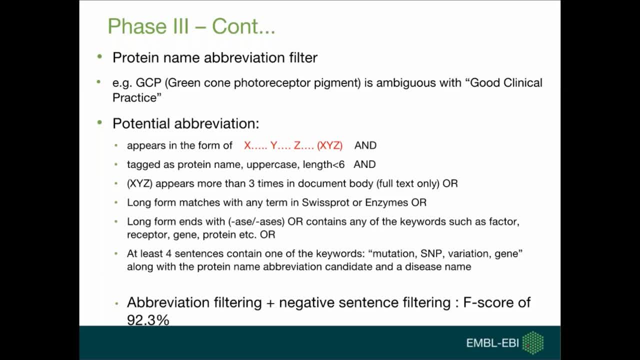 body, Or the long form matches with any term in Swiss prot or enzyme database, Or long form ends with some phrases like is eases, Or it contains any of the keywords, such as factor receptor gene protein. So this is the only clear evidence for us. 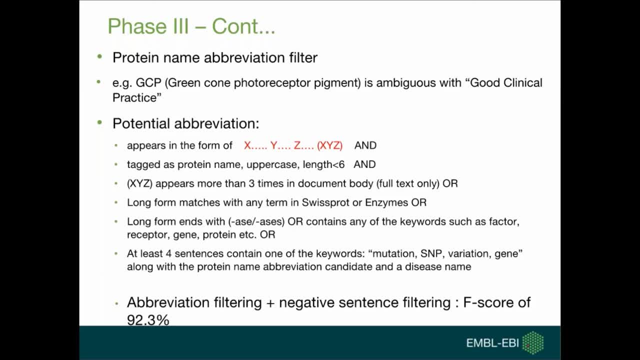 Or at least four sentences contain one of the keywords like mutation, SNP variation gene, along with the protein name, abbreviation candidate and a disease name. We evaluated the performance of our abbreviation filtering and negative sentence filtering steps and we obtained an F score of 92.3%. 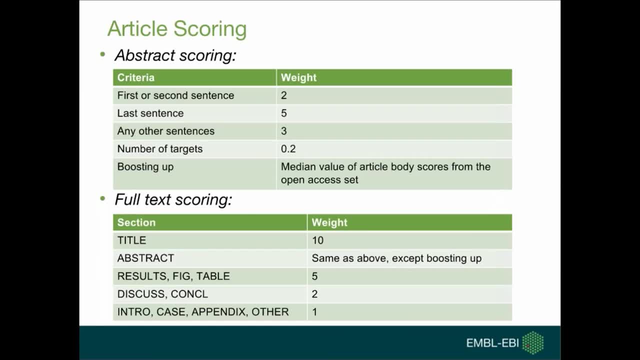 We introduced article scoring in this phase because we wanted to score articles according to the confidences for given gene disease association. Since we have two types of documents, which are abstracts and full text, we implemented two different scoring algorithms. For abstracts, we assigned weights. 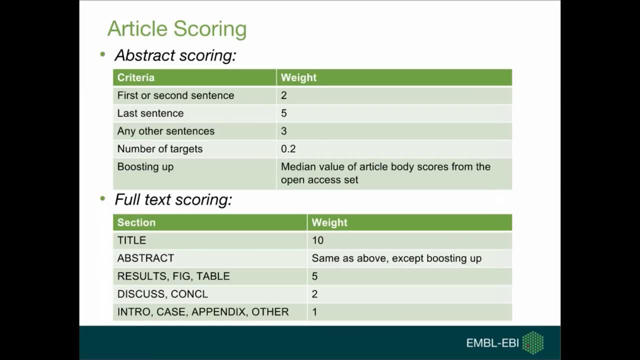 For abstracts, we assigned weights. For abstracts, we assigned weights According to the sentence locations. For example, by our manual analysis we figured out that the lost sentence would be a results sentence. Therefore, we assigned results sentence the highest weight as five. 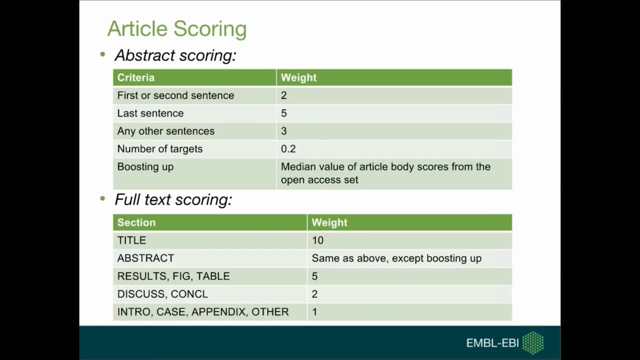 The second sentence or first sentence usually is an introductory sentence, So we assign it the lowest weight as two. We also take into account the number of targets in the article And since article abstracts not in body, we added a boosting up factor to the score. 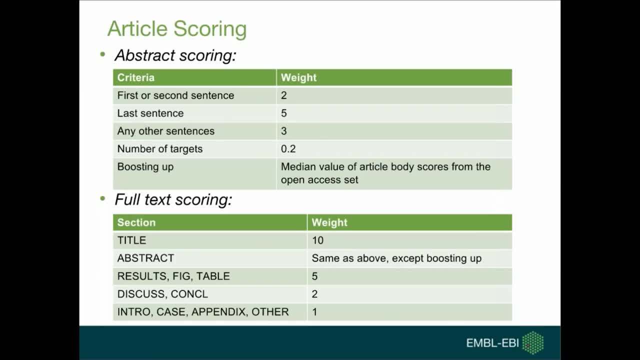 And this boosting up factor is the median value of the article body scores from the open access set that we obtained. For assigning scores to full text articles, we use section information, For example. title would be the most confident part. therefore we assign the highest weight. 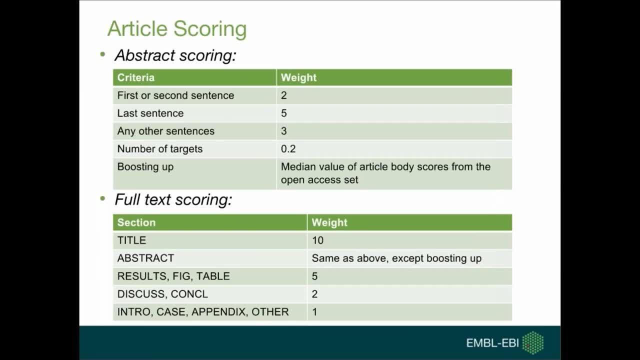 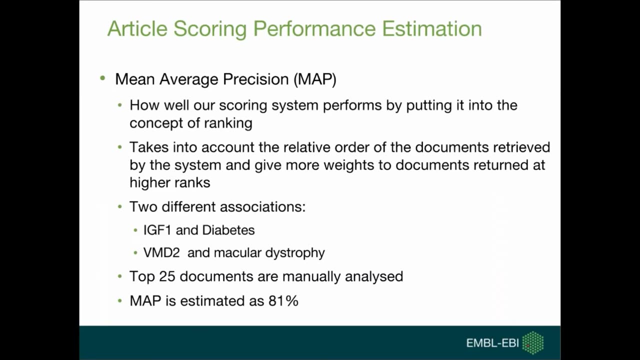 10, to article And we assign the lowest weight 1, to introduction, because introduction usually contains background information And this wouldn't be new and interesting Finding for scientists, Since we introduce article scoring to the system and we assign the lowest weight 1,. 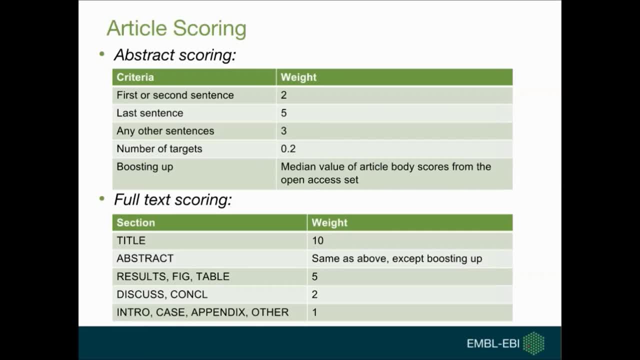 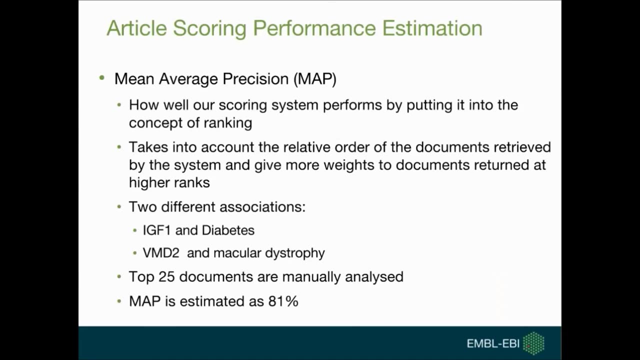 to introduction, because introduction usually contains background information And this wouldn't be new and interesting finding for scientists. Since we introduce article scoring to the system, we needed to switch to another performance metric called mean average precision, And we use this metric. This means it can get out at any time. 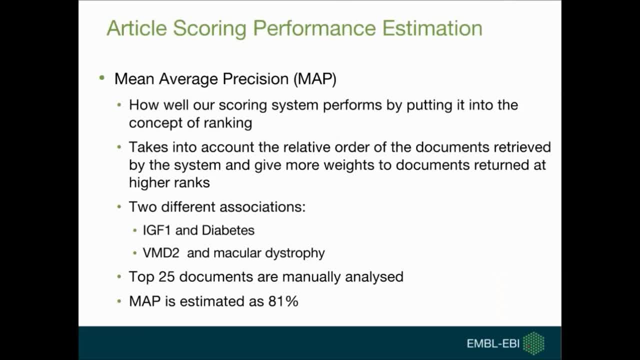 It can bring out any material value UnderOPER frames function publishersли the report values were added to the result And this was our decision. Map takes into account the relative order of the documents directly by the system and gives more weights to document returned at higher ranks. 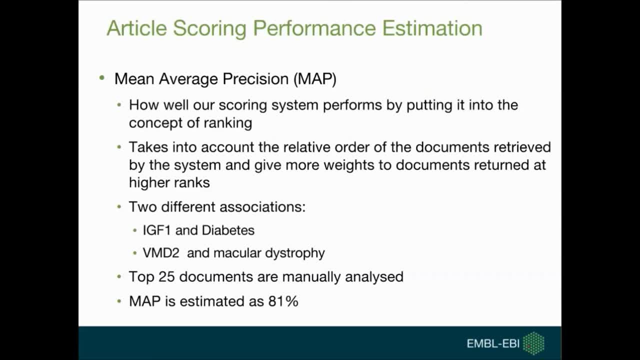 We randomly selected two different associations and used them to estimate the map performance. We selected top 25 documents because we thought that the top 25 documents, that those they would 25 documents- would be the most interesting documents for the user. We evaluate them manually and estimated the map as 81 percent. Now I would like to 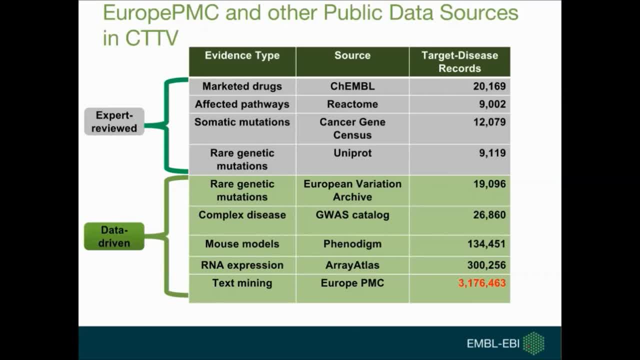 provide some statistics on the data. As I mentioned before, CTTV integrates evidences from different resources. For example, it integrates marketed drugs from Campbell, affected pathway information from Reactor somatic mutations from cancer genes and mouse models from Phenodyne. And, interestingly,